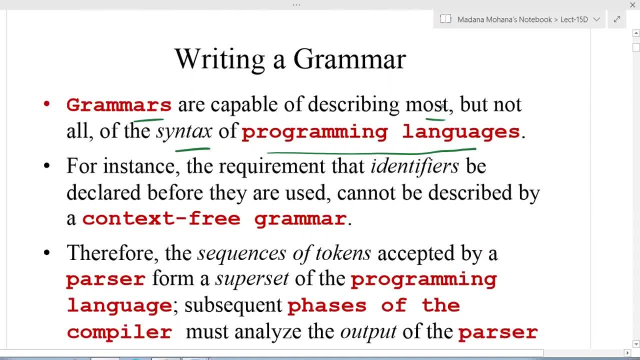 of programming languages, So which are capable of describing most but not all of the syntax of programming languages, So which are capable of describing most but not all of the syntax of programming languages. For instance, the requirement that identifiers be declared before they are used cannot be described by a context-free grammar. Therefore, 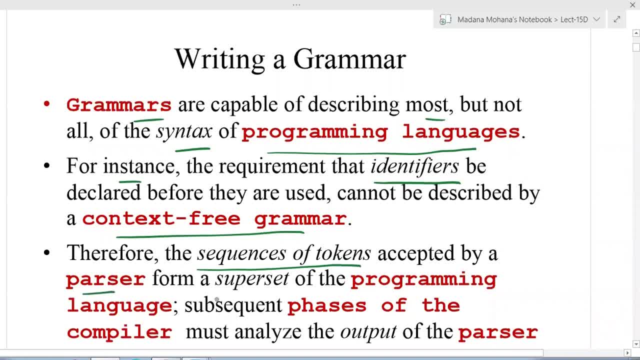 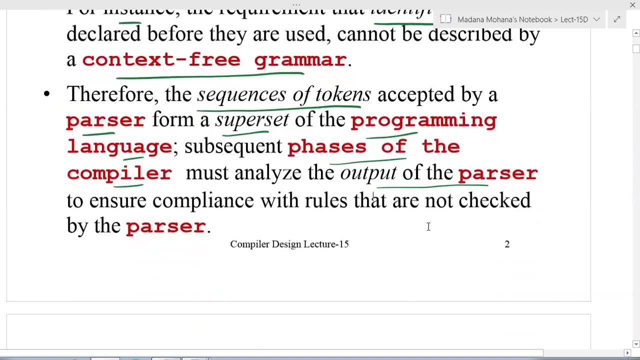 the sequence of tokens accepted by a parser from a superset of programming languages. then subsequent pages of the compiler must analyze the output of the parser. So the sequence of tokens accepted by a parser from a superset of programming languages is called a grammar Finally, which ensures the compliance with rules that are not checked by the parser. 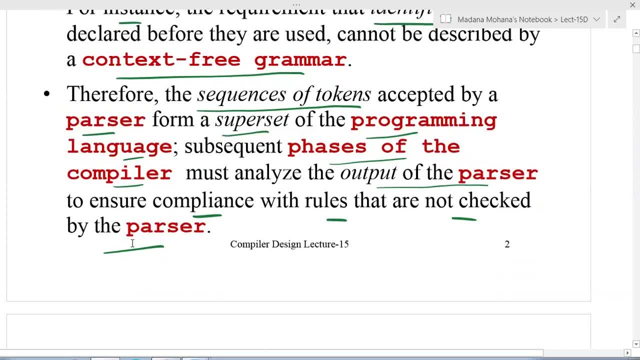 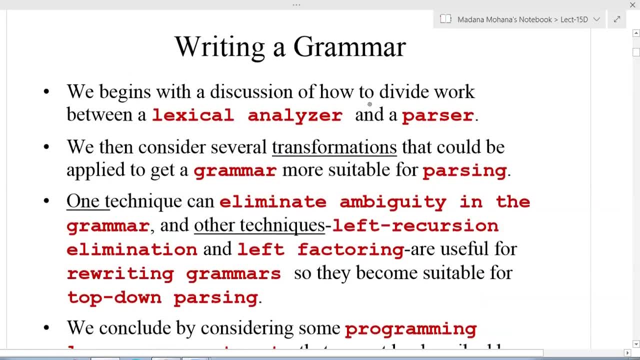 So this is the role of writing a grammar. So here we begin with a discussion of how to divide work between the lexical analyzer, which is the first phase of compiler, and the second phase, parser, of syntax analysis. We then consider several transformations to 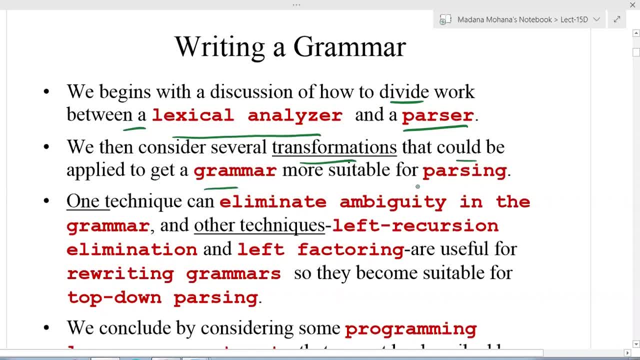 that could be applied to get a grammar which can be suitable for parsing. So one technique can eliminate ambiguity in grammar In formal language and automata theory. this concept we already discussed. same concept used here also. Then other transformations like left recursion elimination. 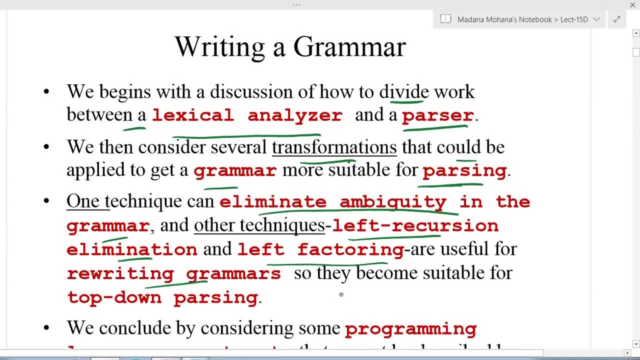 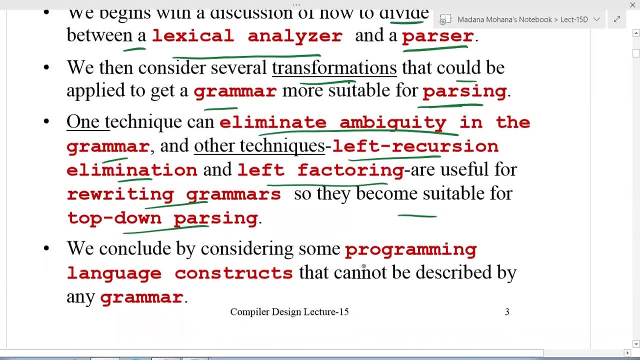 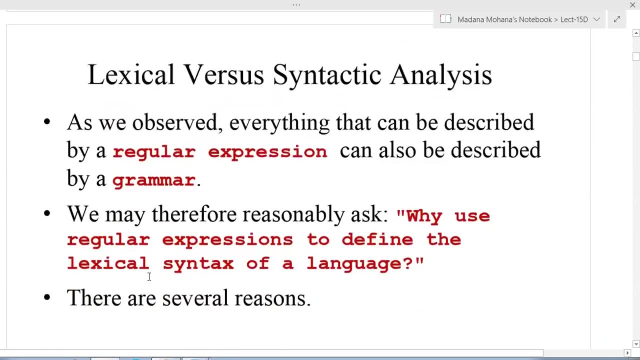 then left factoring, so which are useful for rewriting grammar, so they become suitable for top-down parsing. Then, finally, we conclude by considering some programming language constructs that cannot be described by any grammar. Now, lexical analysis versus syntax analysis or syntactic analysis. 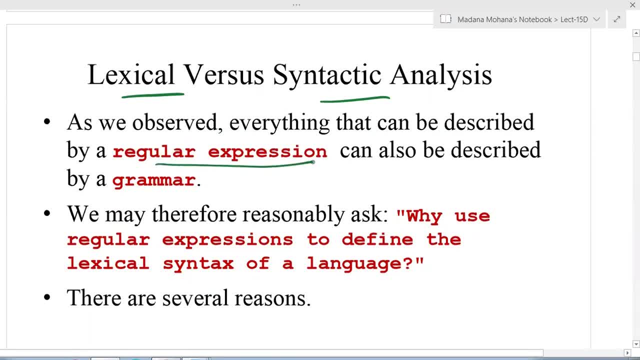 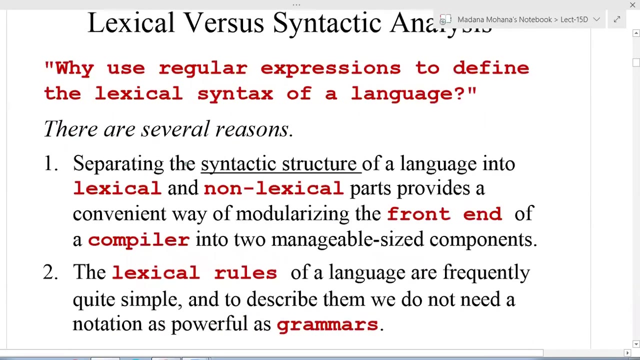 So, as we observed, everything that can be described by a regular expression can also be described by a grammar. We may therefore reasonably ask: why use regular expressions to define the lexical syntax of a language? For this question, there are several reasons. The first reason is separating the syntactic structure. 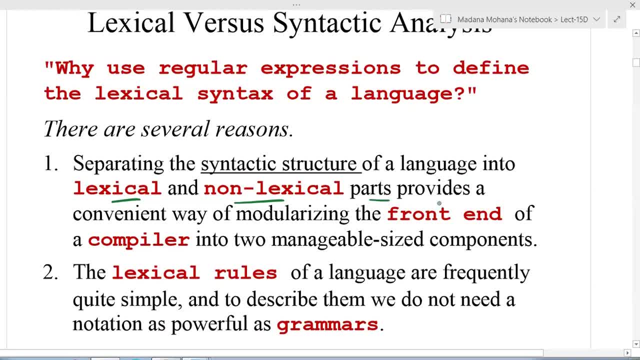 of a language into lexical and non-lexical parts, which provides a convenient way of modularizing the front end of the compiler into two manageable sized components. That is one of the reasons. The second reason is that if you have a language, you can use it to define the syntax of a language. 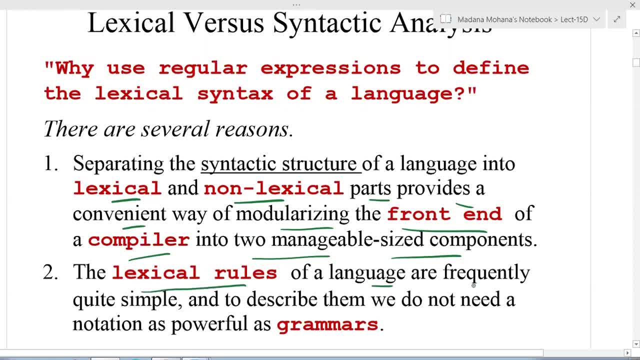 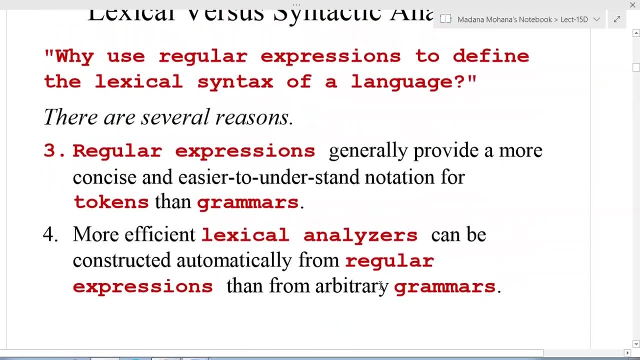 The second reason is that if you have a language, the lexical rules of a language are frequently quite simple, And to describe them we do not need a notation as powerful as grammar. This is the second reason. Then the third reason: regular expressions generally provide a more concise 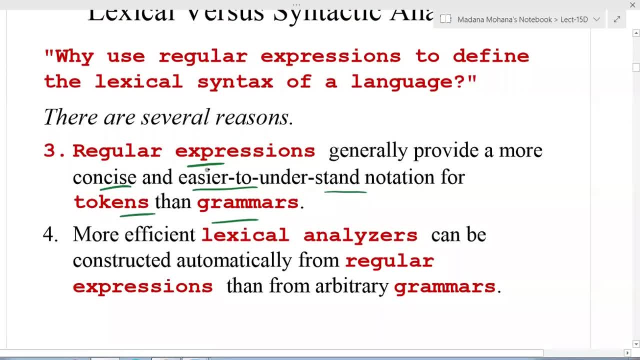 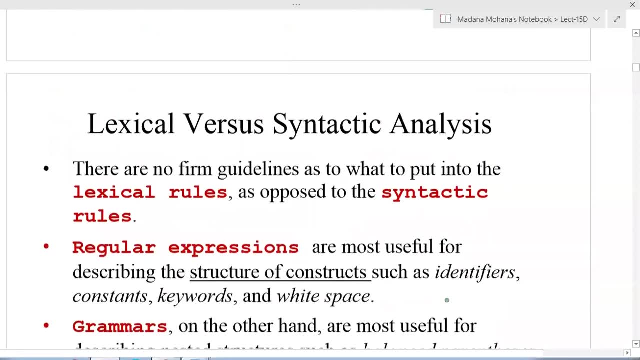 and easier to understand notation for tokens and grammars. This is another reason. Then, finally, more important, this is the third reason: The more efficient lexical analyzers can be constructed automatically from regular expressions than from arbitrary grammars. These are all the several reasons. 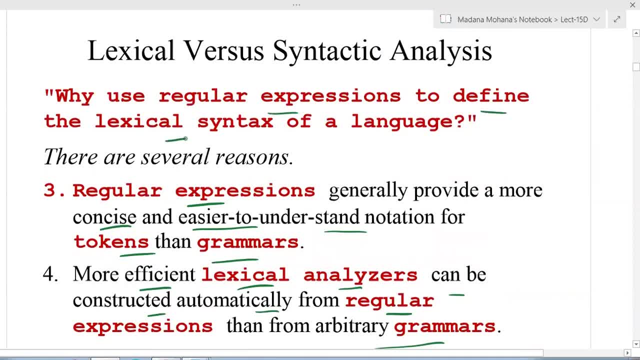 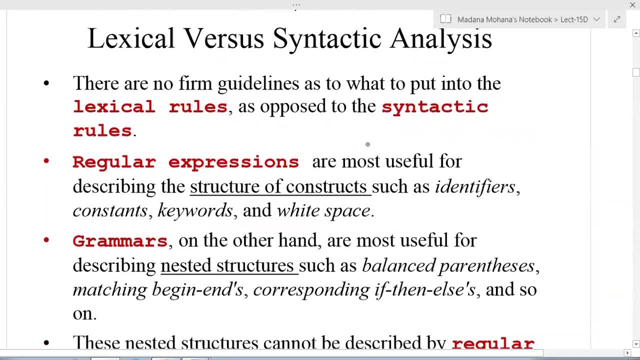 why we use regular expressions to define the lexical syntax of a language. because of these reasons, So this will be done Now. there are no firm guidelines with standard guidelines as to what to put into the lexical rules as opposed to the syntactic rules. 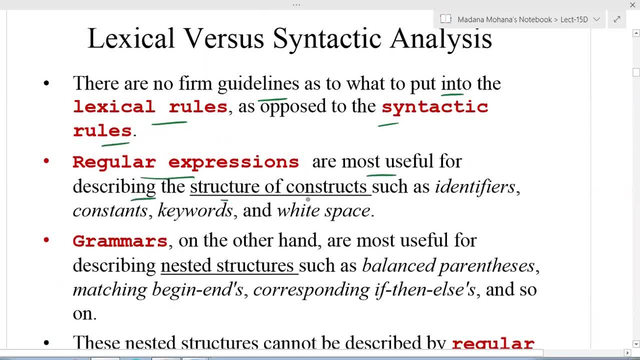 Regular expressions are most useful for describing the structure of constructs, such as identifiers, constants, keywords and white spaces. These are all nothing but tokens. Then grammars, on the other hand, are most useful for describing nested structures, such as the balance references. 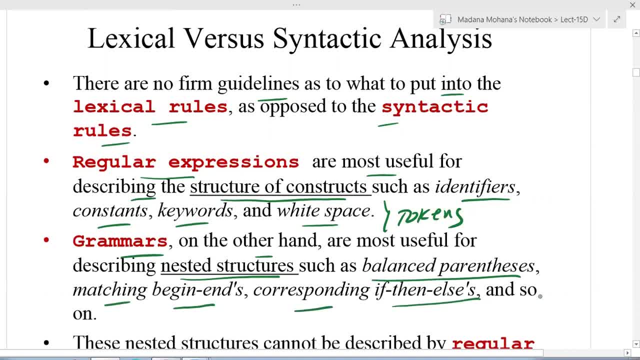 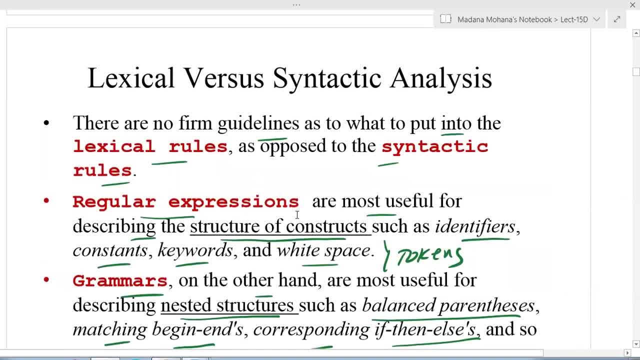 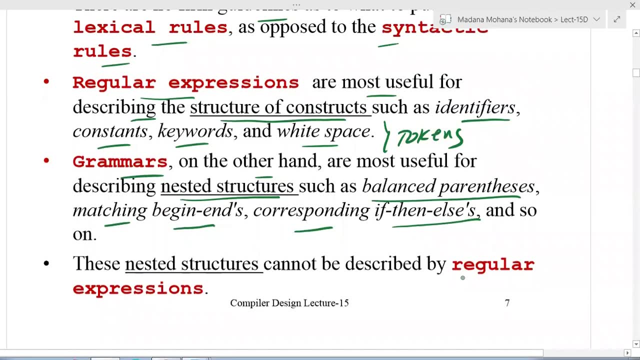 matching begin-ends, corresponding if-then-else, and so on. So these are all the benefits of regular expressions and grammars. Regular expressions corresponding to lexical analysis, grammars corresponding to syntactic analysis- Then these nested structures cannot be described. 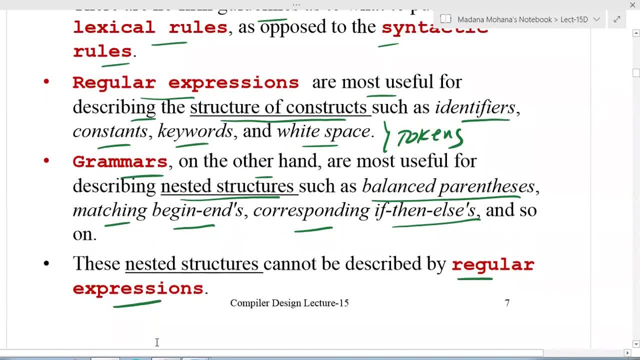 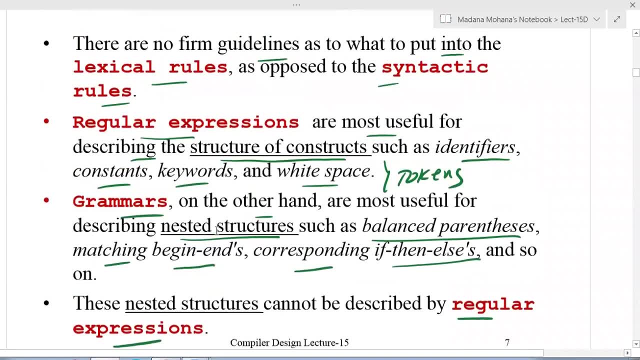 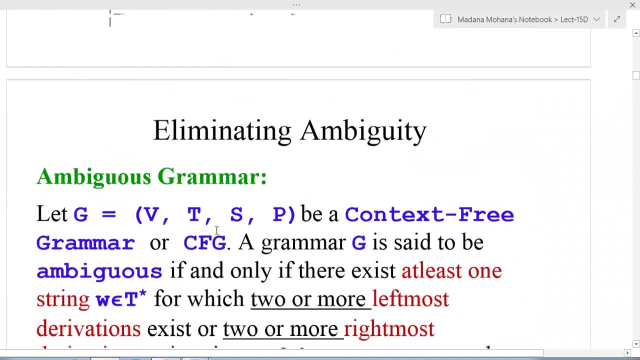 by regular expressions. Whatever the nested structures described by the grammar, those are all not described by regular expression. So these are all the comparisons between lexical versus syntactic analysis, With some similarity solved. Then the first transformation: how to eliminate ambiguity In our previous lecture. 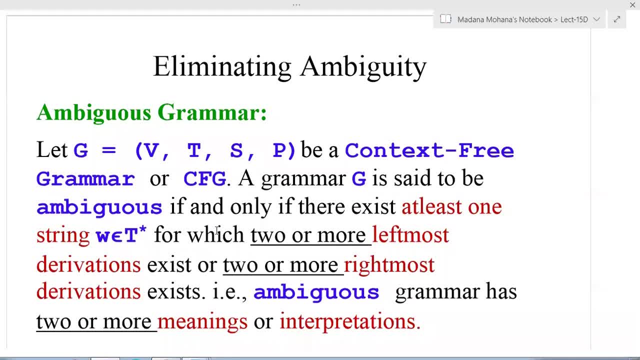 we discussed about what is ambiguous grammar Then how to check whether a given grammar is ambiguity or not. That means for a string. so if it has two or more leftmost derivations or rightmost derivations for a given string, then the grammar is said to be ambiguous grammar. 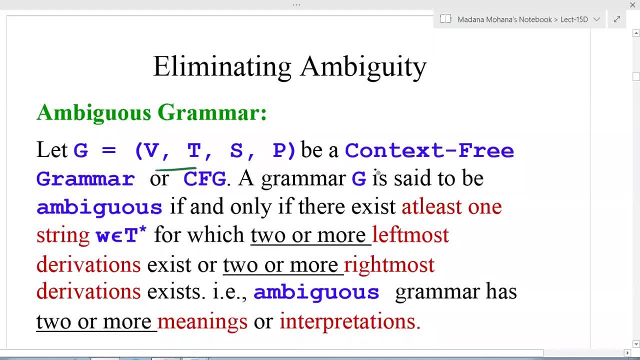 So let us recall the same definition. Let G equal to VTSV be a context free grammar A. grammar G is said to be ambiguous if and only there exists at least one string- W belongs to T closer- for which two or more leftmost derivations exist. 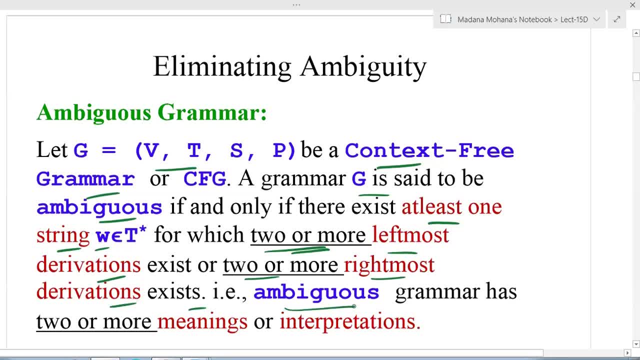 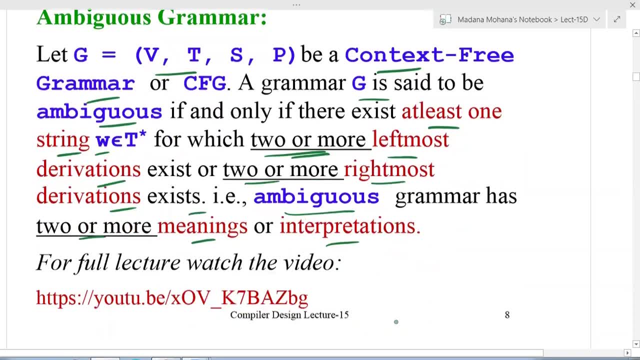 or two or more rightmost derivations exist. That is ambiguous grammar. That means ambiguous grammar has two or more meanings or interpretations. So in formal language and autobiography there are two or more meanings. So in formal language and autobiography there are two or more meanings. 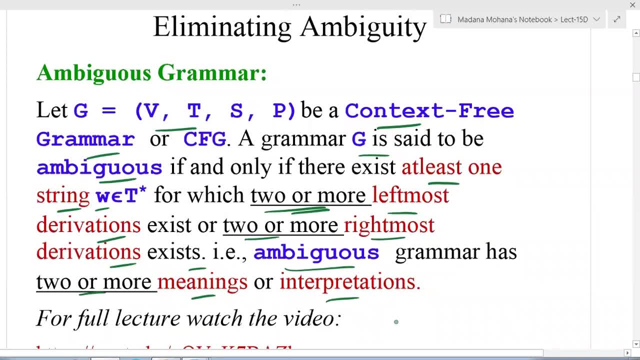 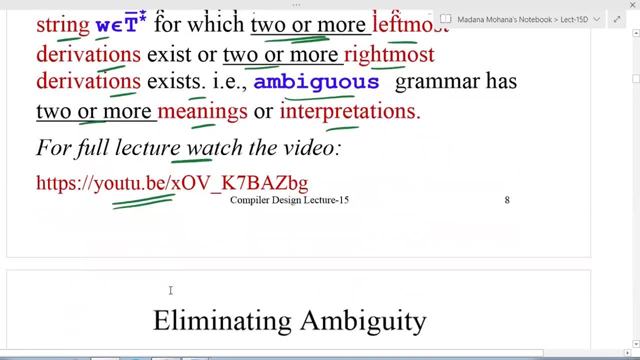 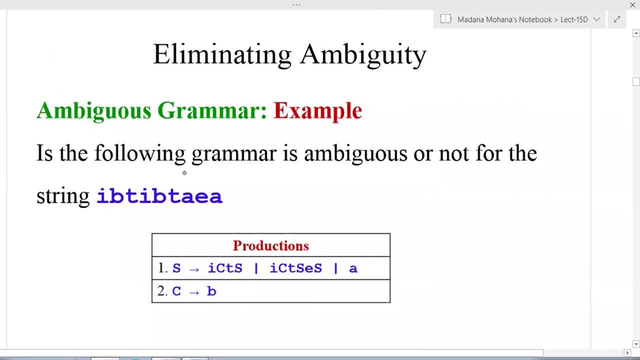 This is the bottom-out of the method theory we discussed about the concept of elimination of ambiguity, For that lecture link is given here. You can go through this for more data. So then let us just start with an example for ambiguity. The question will be like this: 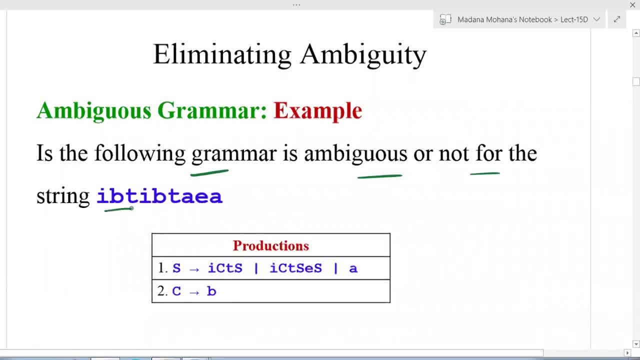 Is. the following grammar is ambiguous or not. for the string IBT, IBTAEA, The productions are given: S derives I, CTS, I CTS, ES or A, then C derives B. all lowercase letters or terminals. uppercase letters are variables or non-terminals, so here: 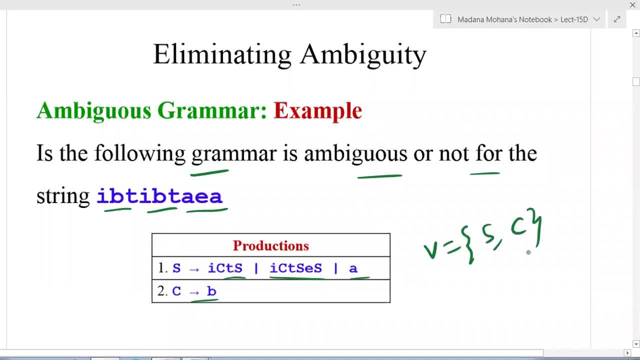 v, equal to capital s, comma, capital c. now terminals are small i, small t, small e, small a or small b. these are other terminals in the grammar g, equal to v, t, s, p. now productions are given here in this table. so now, first we will check with ambiguity, followed by then how to eliminate ambiguity. 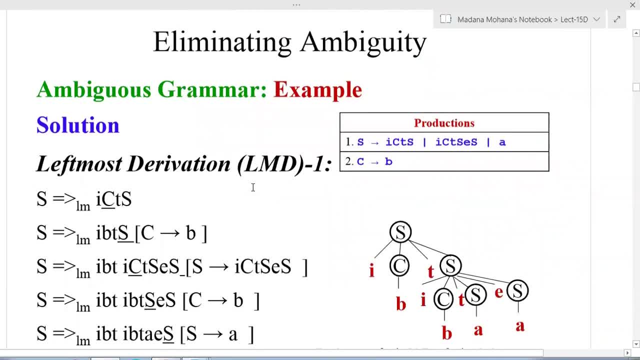 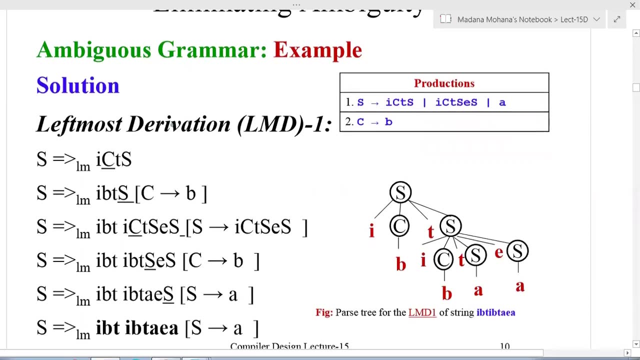 so ambiguity means first you need to construct minimum two leftmost derivations or two rightmost derivations for the given string. then only you can say: the string is, the grammar is ambiguous. so now for the string i, b, t, i, b, t, a, e, the leftmost derivation one. so here, first we have 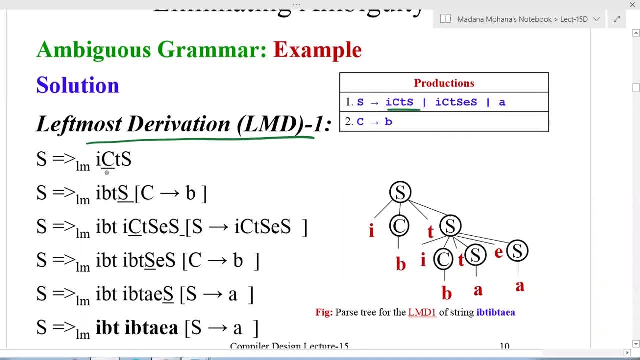 taken the first part of the s production, that is, icts. we have taken then leftmost derivation. every time leftmost variable is substituted, then c is substituted with v here. so then only one variable is there. s is substituted with icts. yes, so then here two variables: s. 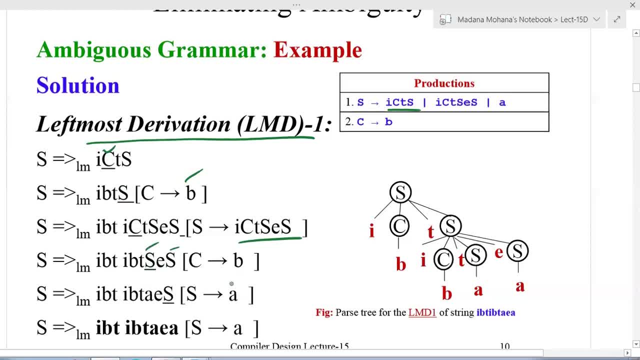 are there. the leftmost s is substituted with a, then finally s is substituted with a. now you can see ibt, ibt, a. so this is the leftmost derivation one. now the corresponding derivation tree is also shown here. so whatever the steps, same steps. you can represent hierarchically: 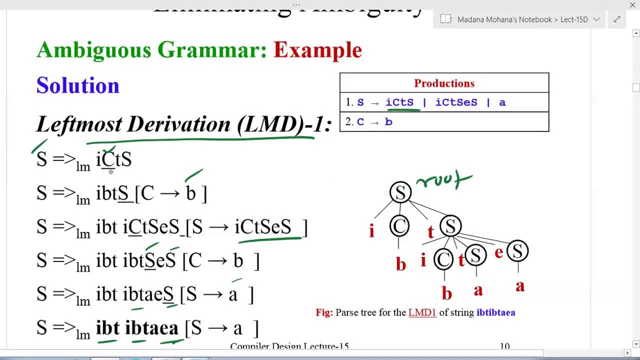 first root is: yes, this is the root. then we have connected ict is from left to right as children's. then all the internal nodes and root are denoted with uppercase letters and represented within circle. Then all leaf nodes consisting of in這一hat has been discuss over, then all the internal 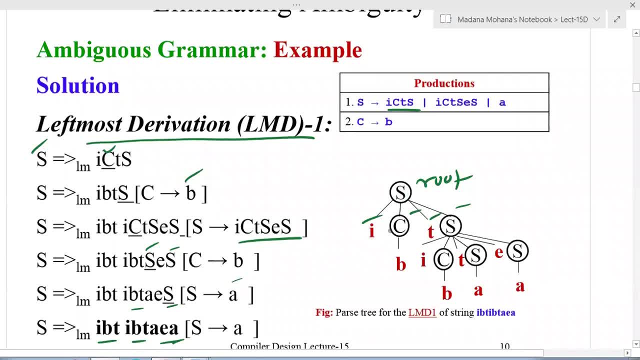 nodes and root is deunited with uppercase letters represented within circle, then all leaf notes, then all leaf nodes consisting of kim and basket terminals- here we can't use circles. now here i is terminal. c is internal node. now here c is substituted with b, then t is a terminal. now s is the variable or non-terminal. s is substituted. 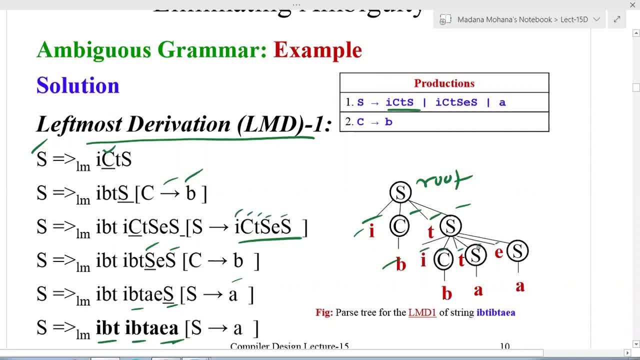 with i c t s e s. so i c t s e s, now all the internal nodes represented with circles. that means which consisting of variables. so now c is substituted with b here, then s is substituted with a here, then again s is substituted with a here. now you can take all leaf nodes from left. 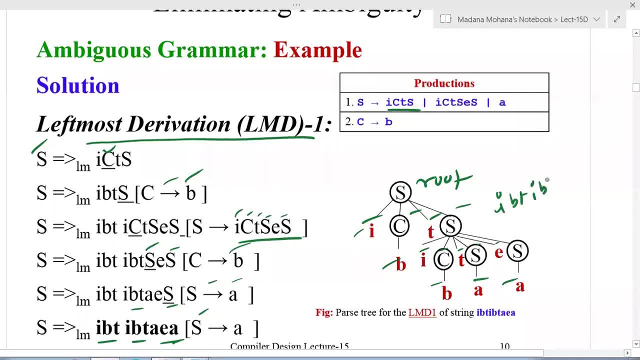 to right, i, b, t, i b, t, a, e, a, from left to right, writing all the leaf nodes from this tree here. this is one, two, three, four, five, six, seven, eight, nine. then you will get your derived string, which is called as yield of the derivation tree are positive. this is the leftmost derivation. 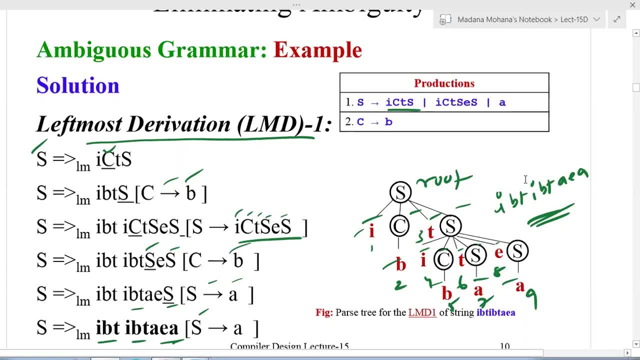 one, two, three, four, five, six, seven, eight, nine, then you will get your derived string, which is called as yield of the derivation tree are positive, this is the leftmost derivation one, two, three, four, five, six, seven, eight, nine for the string i, b, t, i b, t, a, e, a. similarly, let us try to find leftmost derivation two for the same. 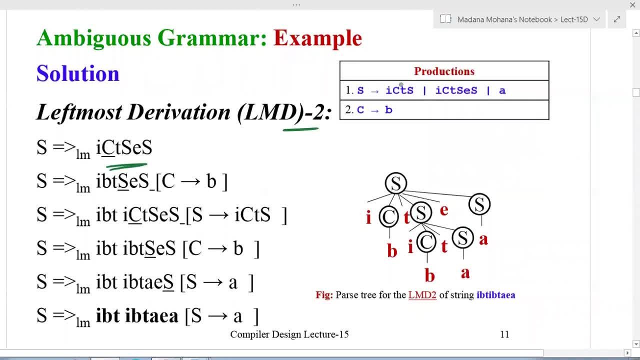 string. now, here we have taken second production of: yes, previously we have taken one, now we have taken second production: i, c, t, s, e, s. so now here three variables are. the leftmost c is replaced with b, then two variables are there, then this s is substituted with i, c, t, s. then again, here we have. 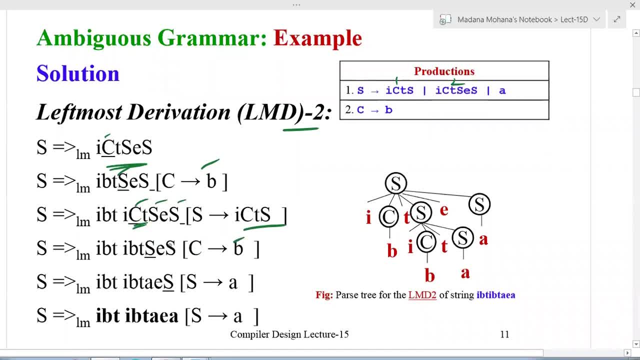 three variables are there. first c is substituted with b. then here two variables are there: yes and yes. first yes is substituted with a, then last yes is substituted with a. now here you can see. we got the same string. so therefore, here for this string, two leftmost derivations are exist. 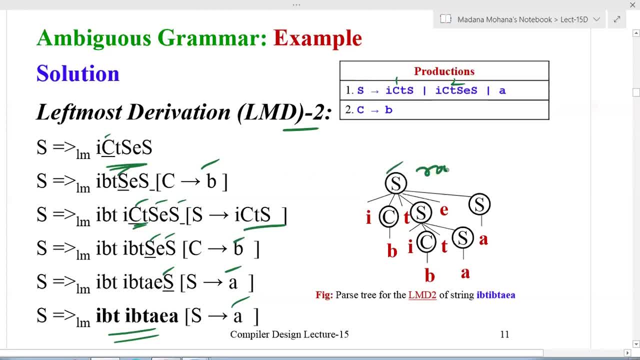 symbol. it's a derivation tree here. first s is the root, then we have connected i c t s e s as children's from left to right to s. so i c t s e s. now c is substituted with b, then s is substituted with i c t s, then again c is substituted with b. 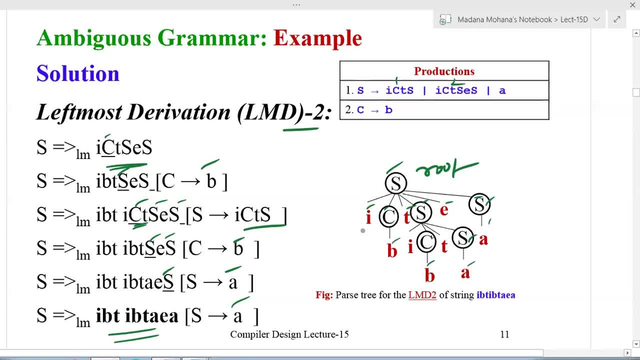 s is substituted with a, then last s is substituted with a again. you can write all the leaf nodes from left to right. now you will get the string. so i, b, t, i, b, t, a, e, a- yield of the tree. so same string is derived. therefore, for this grammar there exist two or more leftmost derivations for the string i. 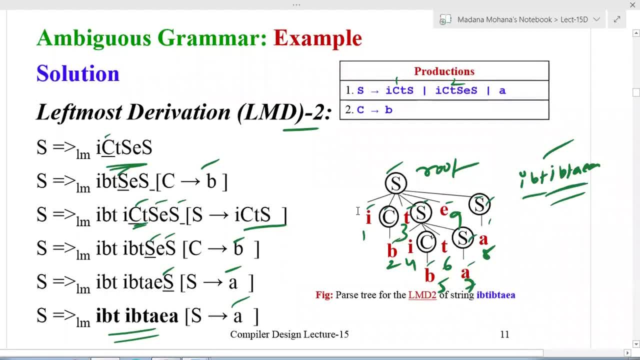 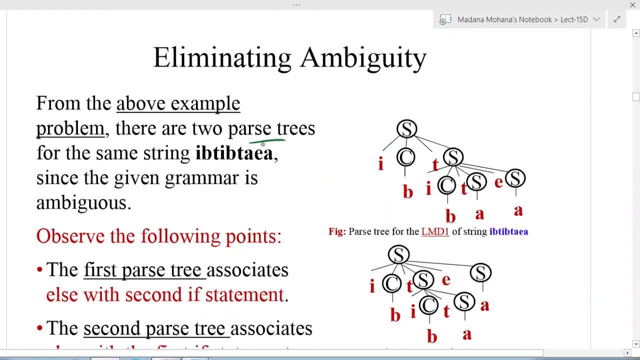 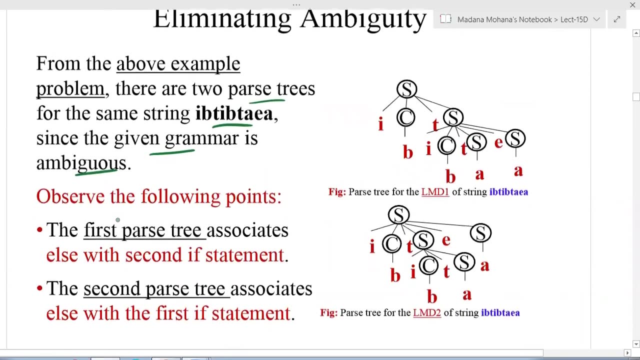 b, t, i, b, t, a, e, a. therefore the grammar is said to be ambiguous. so this grammar is ambiguous. so now, from this example, there are two parse trees from the same string, since the given grammar is ambiguous. here you can observe one point, the first parse tree shown here. here you can see: 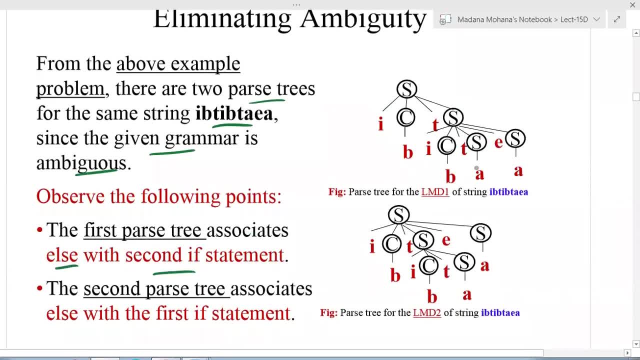 the first parse tree associates else with the second if statement. here you can see the first statement is here. what this, what it contains, ISTS, EAUR, PLS, not there now. here you can see the second statement: i c e t s e s here else. so here else is associated with the second statement, whereas the second 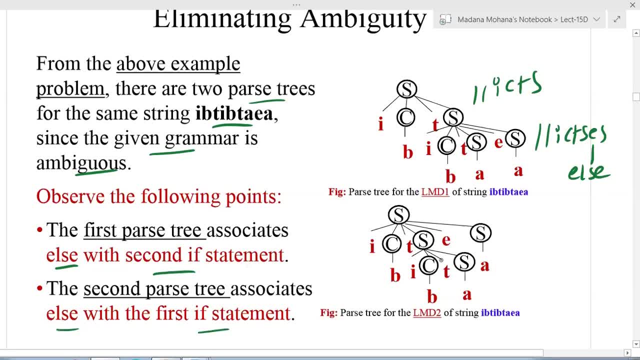 derivation tree. here you can see elis is associated with first if statement. here you can see ICT ES. for here else is associated with first if statement. now, with this one, overnightύ, what will happen in the first two, first three? else is associated with second if statement. 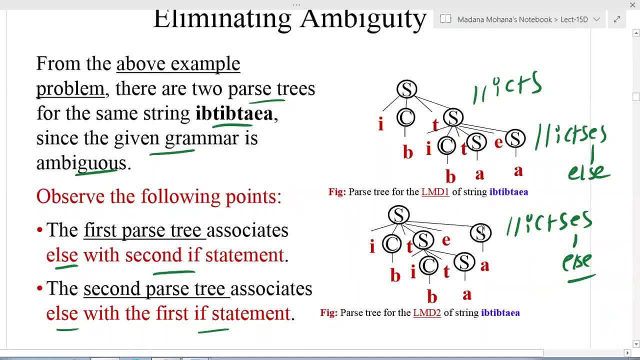 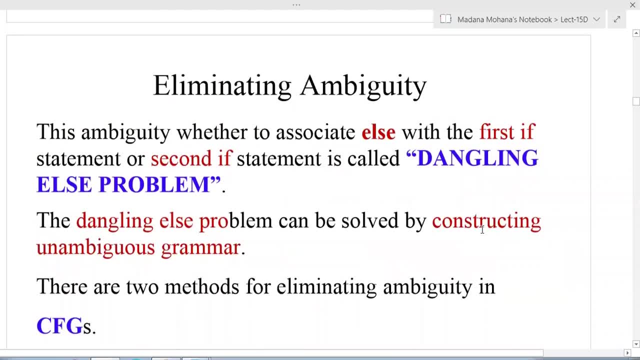 then the second, first, three else is associated with first if statement. now, with this, what will happen? here you can see the ambiguity. this is the ambiguity whether to associate else with first if statement or second if statement. so this ambiguity is called as dangling else problem. so what is the dangling else problem in if then else case? so else is associated with. 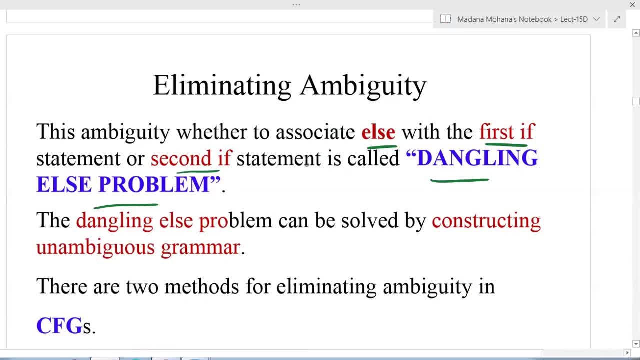 first if statement in one case, then else is associated with the second if statement in another case. now which one needs to be considered. so this problem is called as dangling else problem. so how to solve this problem? by eliminating ambiguity for this grammar, by constructing unambiguous grammar. so the dangling else problem can be solved by constructing unambiguous grammar. 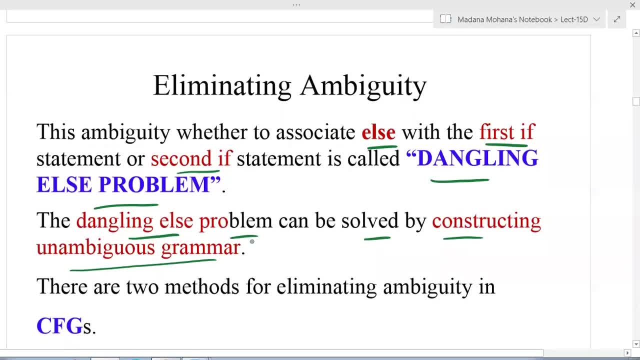 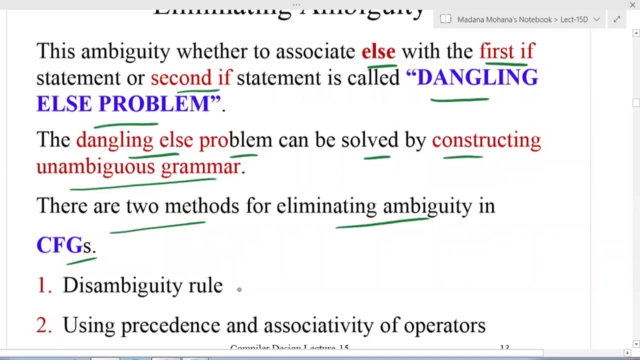 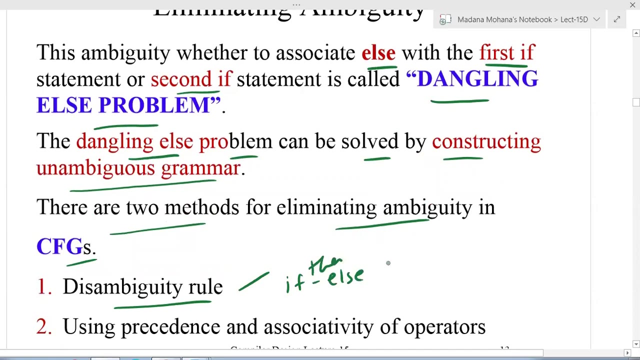 so that means by constructing unambiguous grammar for the ambiguous grammar. that means we have to eliminate ambiguity. so there are two methods for eliminating ambiguity in context-free grammars, as we discussed in formal language and automata theory, same methods. the first one is this ambiguity rule. this we can apply for if then else, if then else statement problem. then second method, using 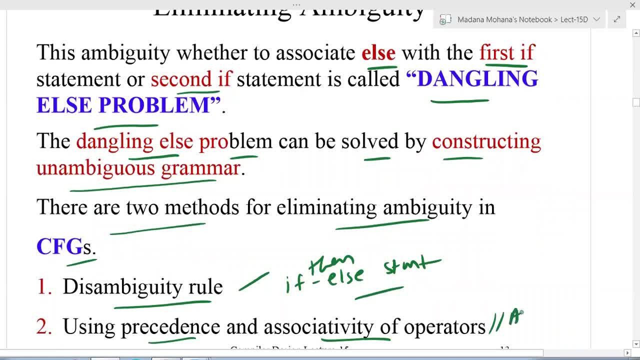 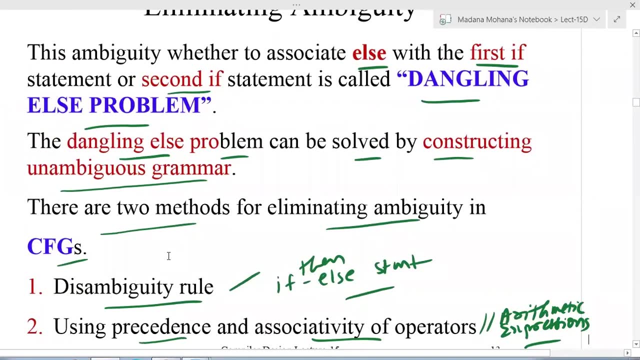 precedence and associtivity operators. this you can apply for money expression grammar where automatic operators are included, whereas any grammar with if, then else else combination, use this ambiguity rule. any grammar which is combination of automatic expressions, you can use precedence and associativity of operators. now we will see one by one. first let us consider the same example: eliminate ambiguity. point goes to such a scene. we would follow the same example: eliminate ambiguity. the first action side of this can be looking for vice, that is времени, all gamification terms, any grammar with Rim match you will have an opposing am chuyure. but when you would be using precedence, these probabilities would子il σαςy pair separ, madam ye u t disciples. now we'll see one by one. first ledgers: concept of the same example: illuminate ambiguity. 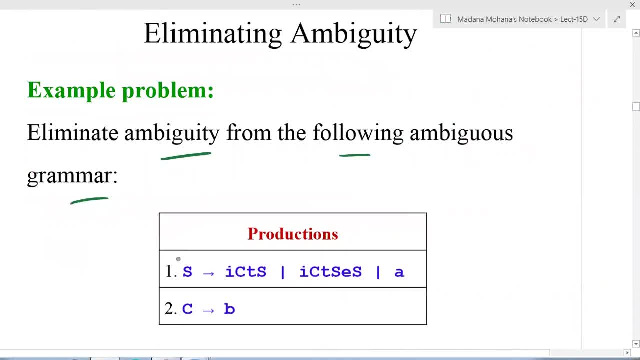 first let us consider the same example: eliminate ambiguity. so if you need to say straight outек smartoganic in the practice across we have here. Eliminate ambiguity from the following grammar: ie S-D-S-I-C-T-S or I-C-T-S-E-S or A, then 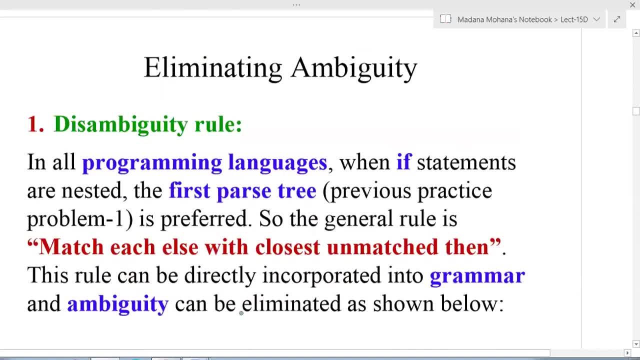 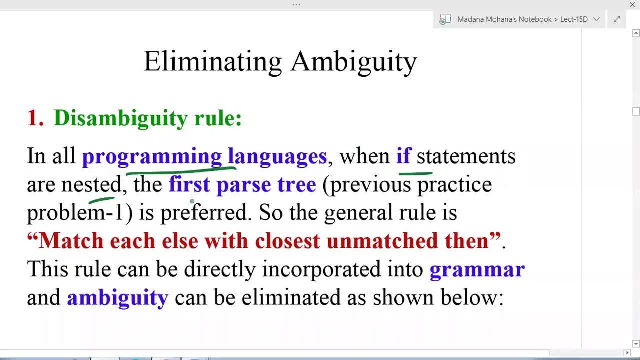 C-D-S-B. Same example, what we discussed now. Now, by applying disambiguity rule. so in all programming languages when if statements are nested, then the first parse tree in the previous example is preferred. So the general rule is: match each else with closest unmatched. then 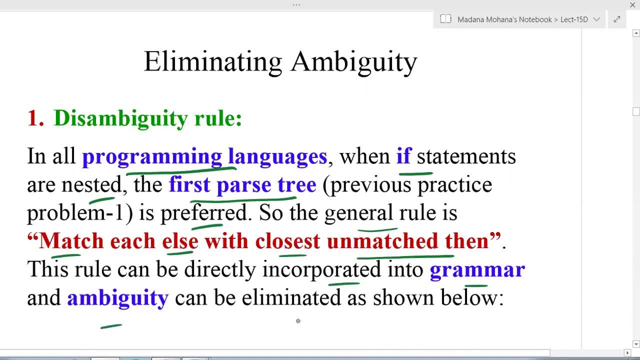 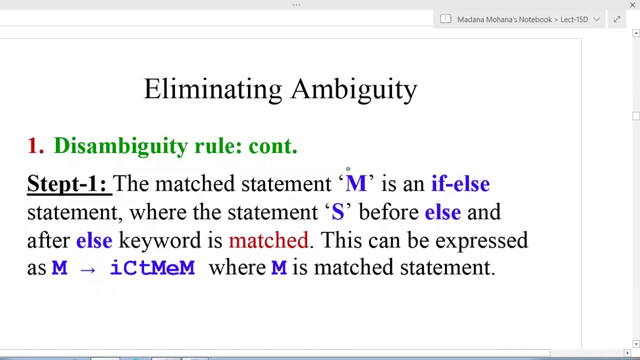 This rule can be directly incorporated into grammar and ambiguity can be eliminated as shown below. So every time we can consider this rule, match each else with closest unmatched then statement. Now step one, the match statement. let us say capital M, which is an if-else statement. 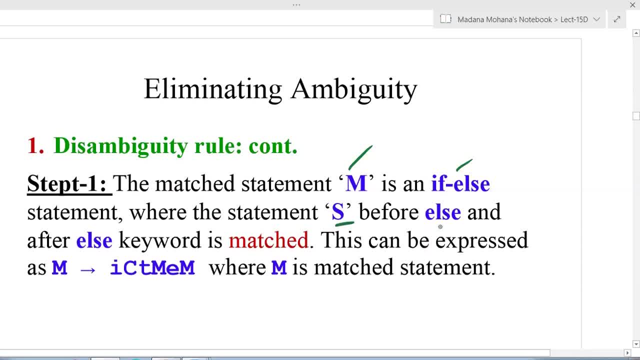 simple if-else statement where the statement yes, before else and after else keyword is matched. So this can be expressed as: M derives actually the original production, S derives I-C-T-S-E-S. Now here we are, defining the statement as matcher statement. 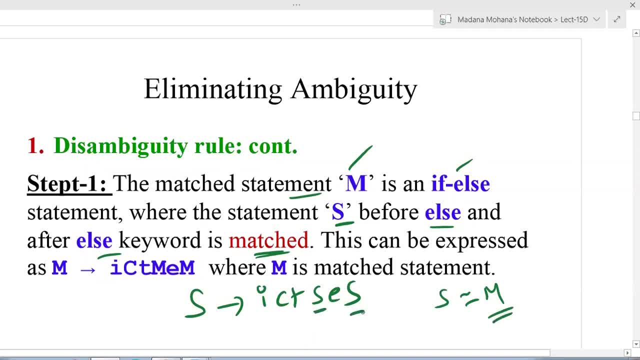 So this matcher statement- before else, after else, now this is else- should be the matcher statement. Therefore, now the statement is replaced with M here. Before else, again, S is replaced with M. After else: S is replaced with M. Therefore, 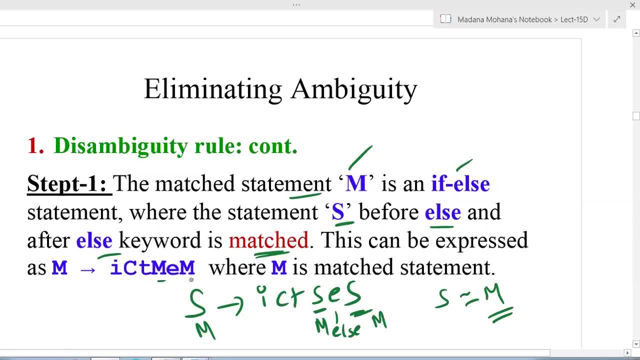 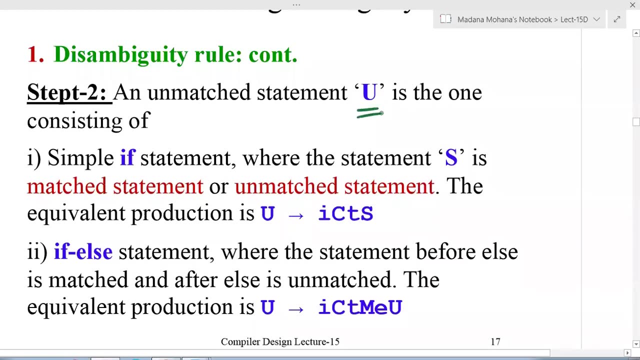 now this will become M derives I-C-T-M-E-M. So this is obtained like this, by taking matcher statement before else, after else. That is step one, Then step two, an unmatched statement. let us say, capital U is the one consisting of: 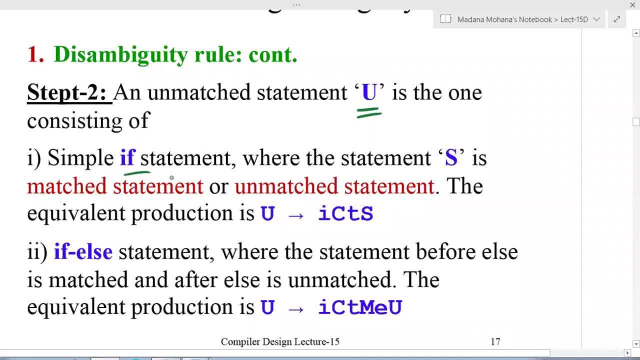 there are two cases for unmatched statements. First one is simple: If statement where the statement S is matched or unmatched statement, therefore the equivalent production is U derives I-C-T-S. So here S is either matcher statement or unmatched statement. That's why directly we have taken S only. 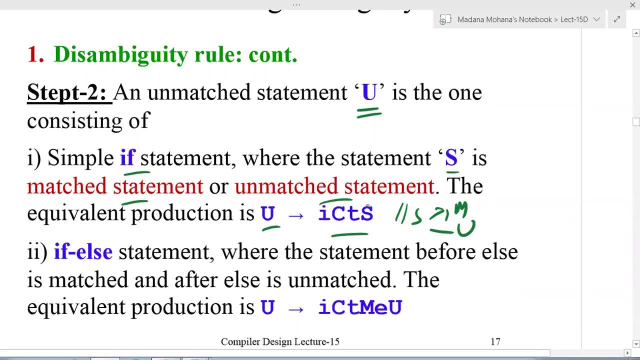 Here two combinations are there, So two at a time. we can't substitute simply S. Then S is defined with matched or unmatched statement, Whereas second case, if-else statement, where the statement before else is matched or unmatched, then after-else is unmatched. 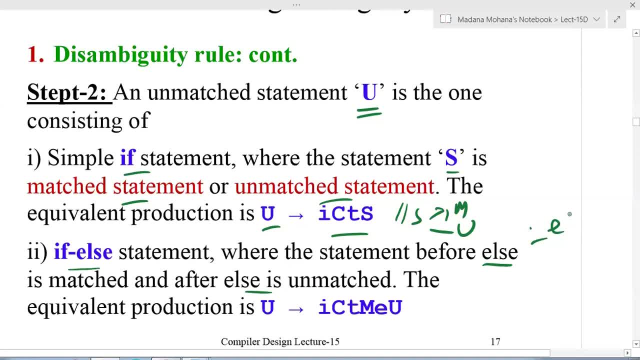 So before-else is match, then after-else is unmatched, M-U. So then the equivalent production is: U derives I-C-T. Now this is else: before-else a matched statement, then after-else unmatched, the statement, So M-U. 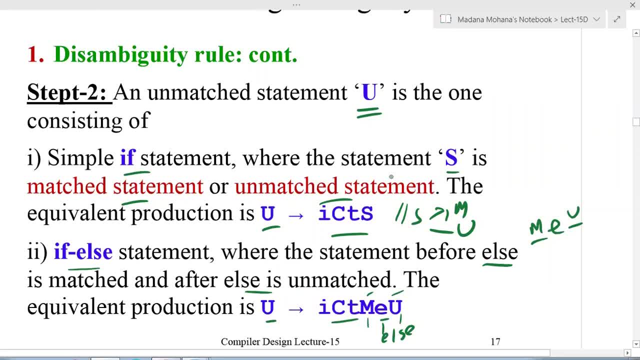 This is the second case. Now for step two. you will have two cases: U derives I-C-T-S and U derives I-C-T-M-E-U. So here for the second case. you will have two cases. Now for step three. you have two cases. 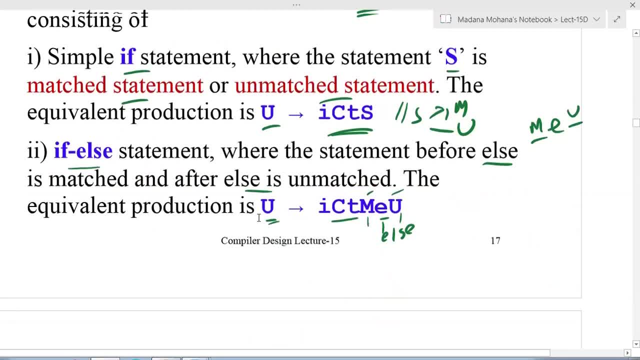 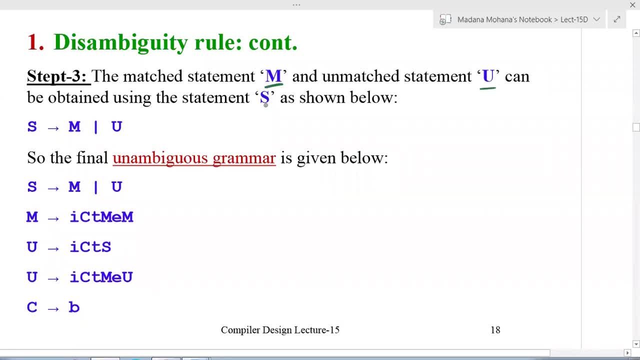 u. two productions are there in this case. then, coming to step three, the match statement m and unmatched statement u can be obtained by using the statement yes combination of these two, as shown below. therefore, s derives m or u. now, in step one, we obtained one production for m. 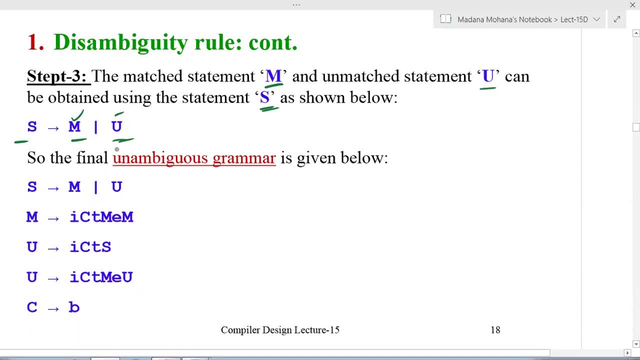 in step two, we obtained two productions for u. now you can write on this production. therefore, the final unambiguous grammar is given below: s derives m or u, first production. now, what is m? in the first step? we obtain m. derives ict mem, then u. in step two, we obtain two productions. 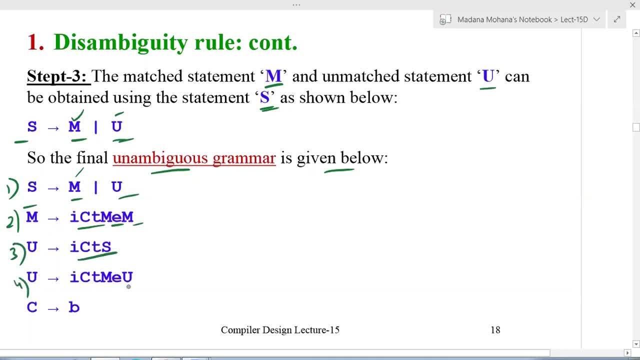 so u derives icts, then u derives ict meu, then c derives b. so no changes in this production as for the given original grammar. so therefore, now this is unambiguous grammar, an ambiguous grammar. so here we applied this ambiguity rule. so for if, then a statement. 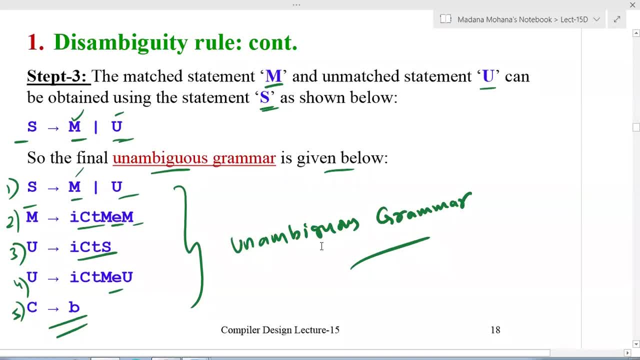 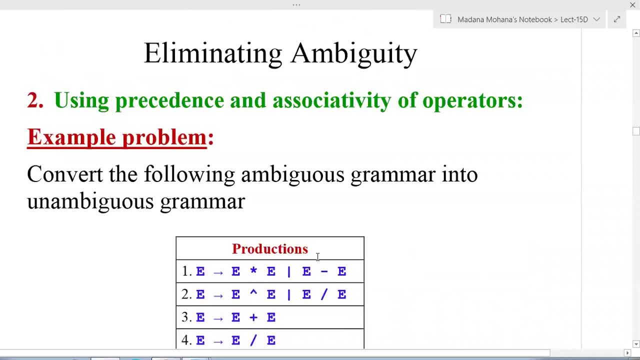 this is the equivalent grammar, after eliminating ambiguity. this is method one, which is called as this ambiguity rule. then, coming to second method, so using precedence and associativity of operators, so in this case the grammar consisting of arithmetic operators, that means automatic expression. so convert the following ambiguous grammar into unambiguous grammar. here you can see what the 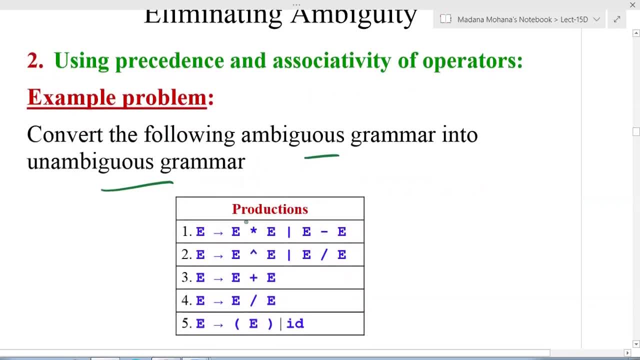 grammar consisting of the productions which are combination of automatic expressions. here e stands for, e stands for expression, then the operators here into: that is multiplication minus, this is subtraction, this is power exponent, then this is divide, then this is automatic addition, then again here. this is repeated, here not required. 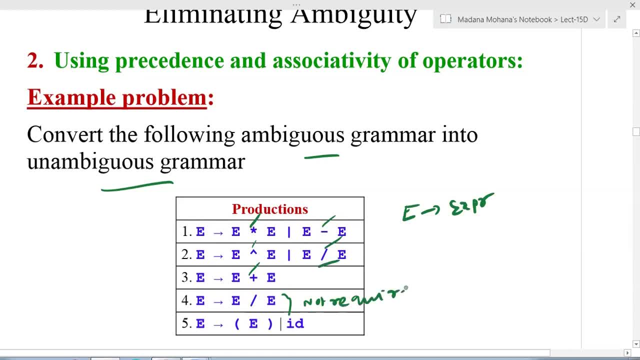 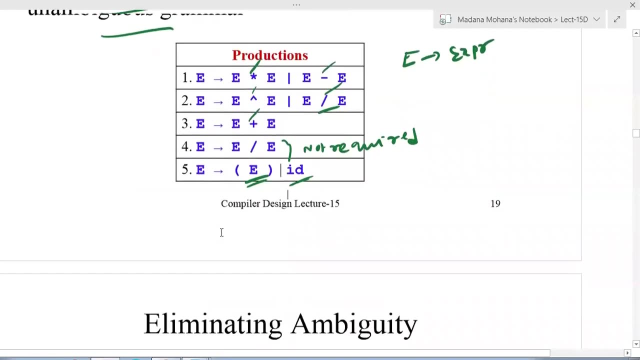 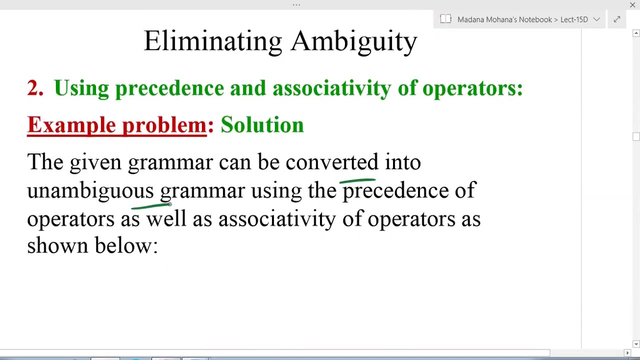 so already division taken here. so now the expression within parentheses then, are identified. so now, using the concept of precedence and associated associativity of operators, here we can eliminate the ambiguity of this kind of grammars. now let us come to the solution. the given grammar can be converted into unambiguous grammar using the precedence of operators as well. 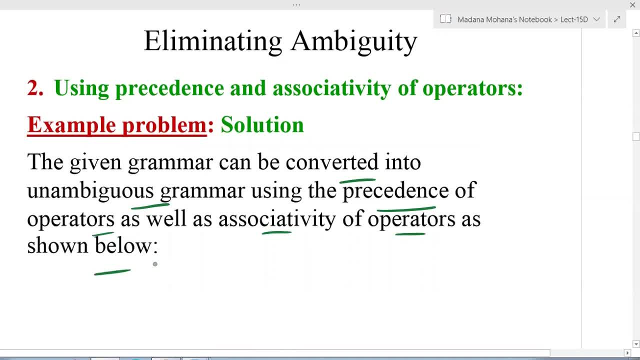 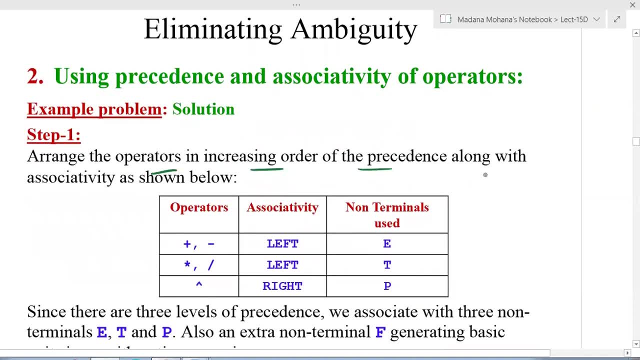 as associativity of operators. so we have picked the precedence operators as shown below. here what you have to do, step one: arrange all the operators in increasing order of the precedence, along with associativity, as shown below. so that means first we have to list the least precedence operators, so in the given grammar plus. 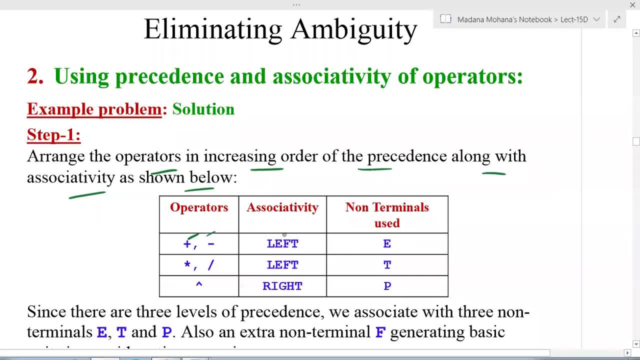 and minus having a least associativity. that means precedence. so now these are all left associative. that means the evaluation can be done from left to right. now we for this a non-terminal E. for this substitution, The next highest precedence is into and divide. Both are all left associative. For these productions we will use the variable T. 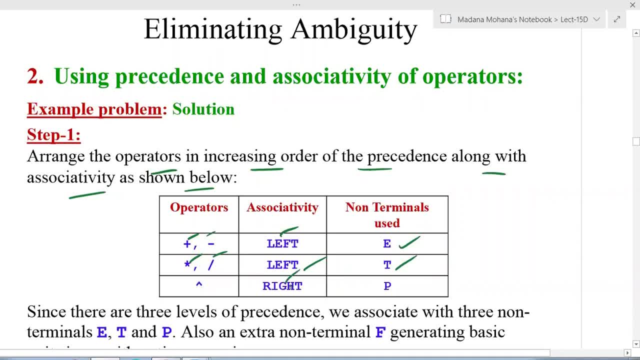 The next one is exponent. It has right associative, So right side evaluation. For this we will use the non-terminal P. So since there are three levels of precedence, we associate with three non-terminals: E, T, P. Also an extra non-terminal F is generating the basic units in arithmetic expressions which 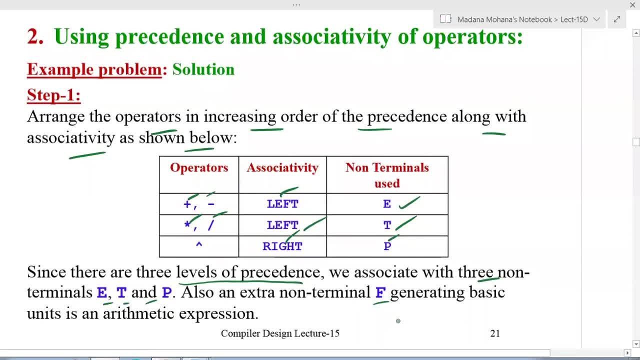 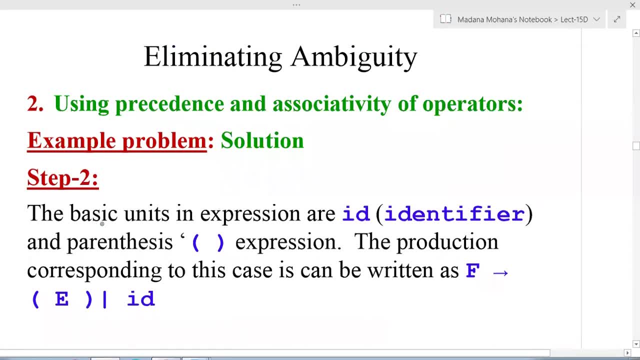 are in F production. F' within parentheses are id. Now move to step two Here. first we'll consider the basic units. The basic units in an expression are id identified and the parentheses that is expression. Then the production corresponding to this case can be written as: 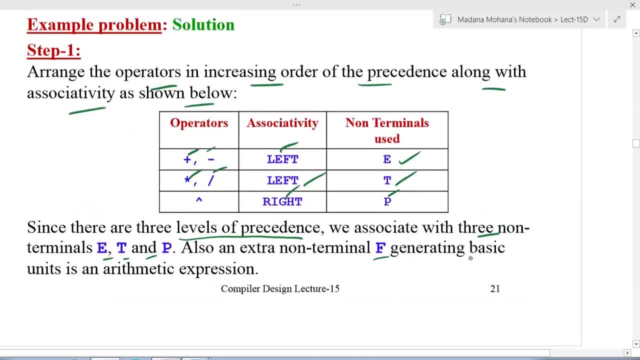 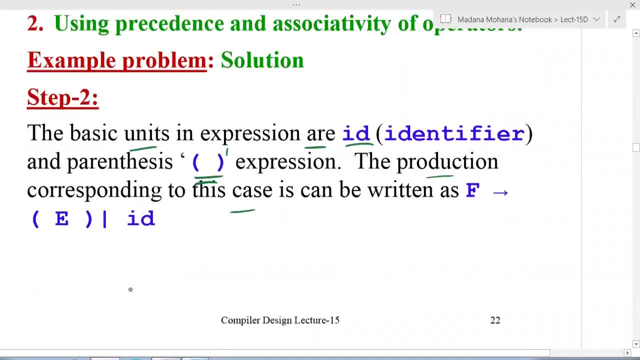 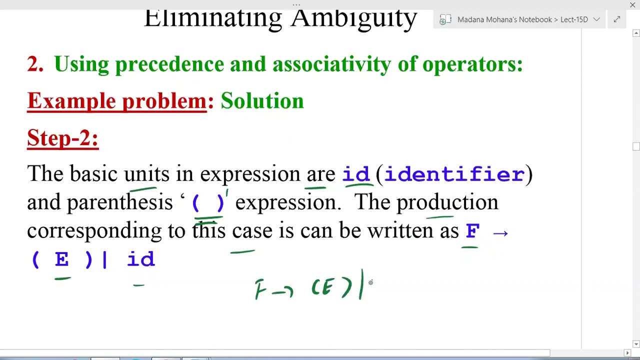 for this we introduced F as the variable, So an extra non-terminal F generating basic units in an arithmetic expression. Therefore, F derives, F derives E. within parentheses are id. So now this is the production which consisting of basic units. Next highest precedence is exponent. 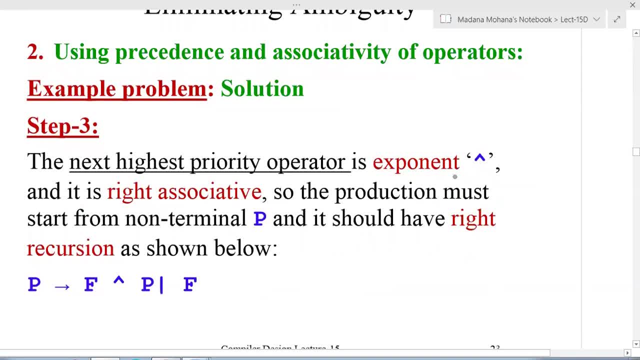 That you can consider here. The next highest priority operator is exponent and it is the right associative. So the production must start from non-terminal P. For this we introduced P as the non-terminal and it should have right associate, right recursion. That means this: 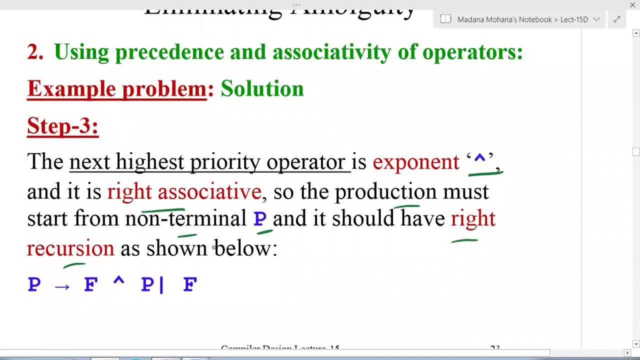 should occur in the right hand side of the exponent operator. So now here P derives F power, P. Actually P power F, F, P is right associative. That's why this should be placed after the operator. That means right side of this operator. So F power P. 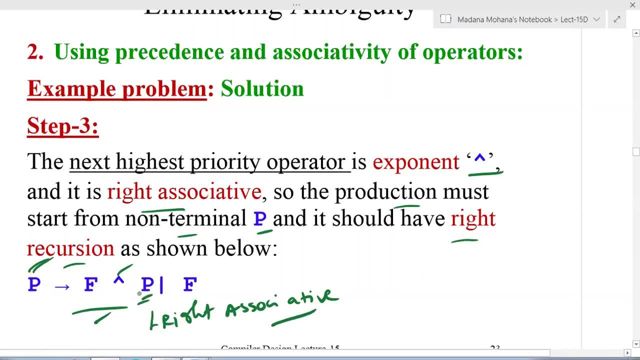 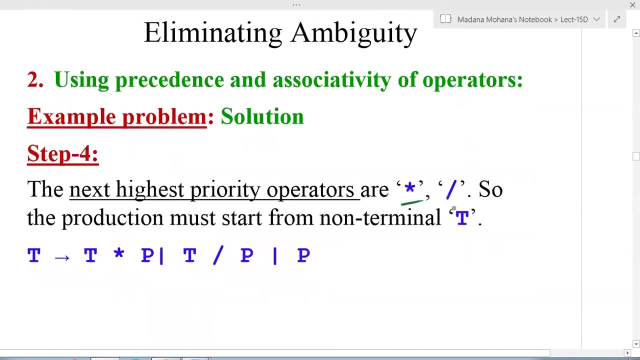 Or F. So these are all P productions. F we know in the previous step. Then next highest priority operators can be derived from P, Starting with the other non-terminal what we introduced. The next highest priority operators are into divide, So the production must start from. 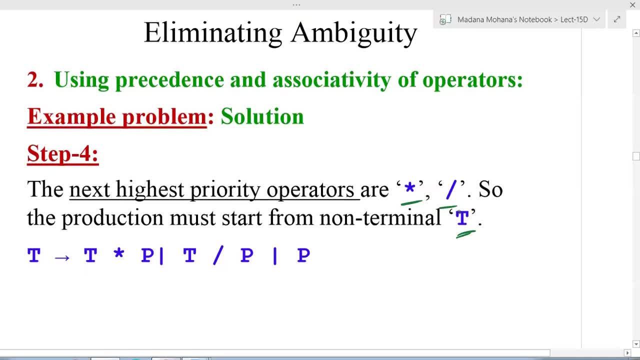 non-terminal T which is left associative. It should be occurred before the operator. That means left hand side of the operator. So now T start with T, derives T into now in the previous one, P, Or then divide Why? Because two operators we have consistent T by P. 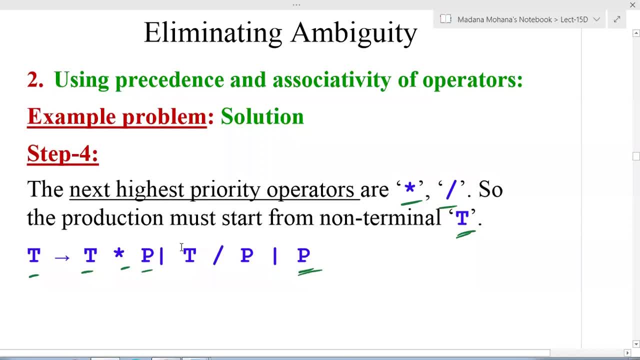 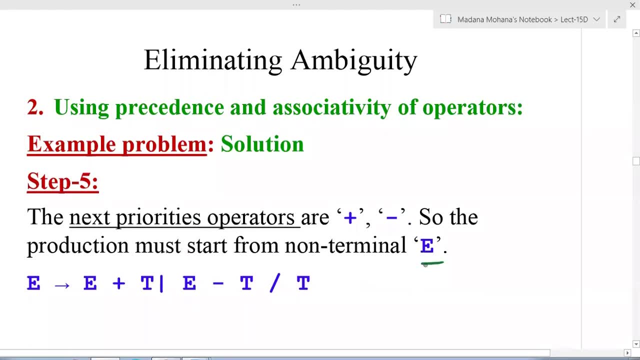 Then R, P. So next priority operators are plus and minus. These are all the least priority So now. so the production must start from non-terminal E. So here this is also left associative. It should be occurred before the left hand side of the operators. Now E derives. 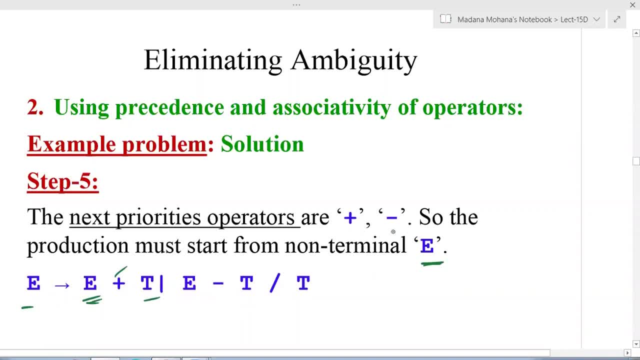 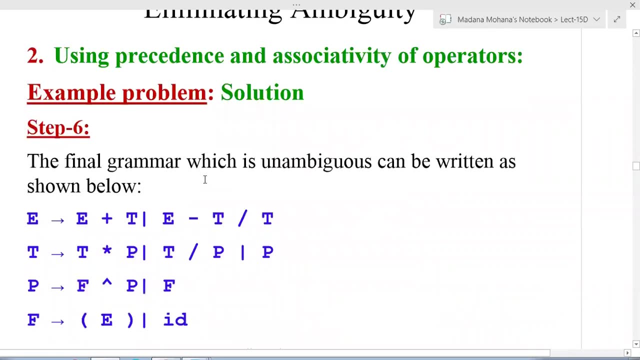 E plus T, So left side it is placed. Then next operator is minus E derives E plus T, E minus T R T. So now see all the group of operators are included. So now we have to combined all the productions starting with the starting variable. Here starting variable is E. 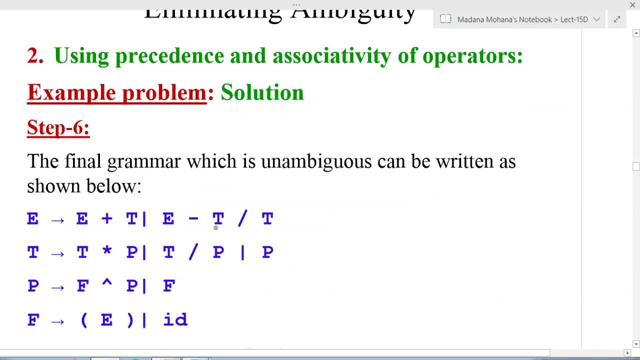 So with E all, you can write down the final productions. The final grammar, which is unambiguous, can be written as shown below, That is, E derives E plus T Or E minus T R T. First we have started with starting variable E, Then here, what is new to? 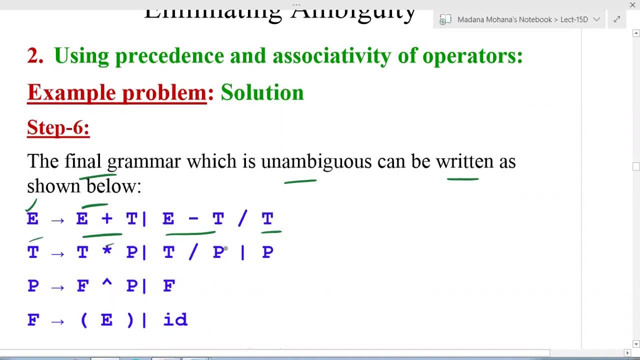 t is new now. introduce t productions. t derives t into p or t by p or p here. what is new? p is new. write down p productions. p derives f power, p or f here. what is the new? production f now. f derives e within parenthesis or id now. this is unambiguous grammar, after eliminating ambiguity using the: 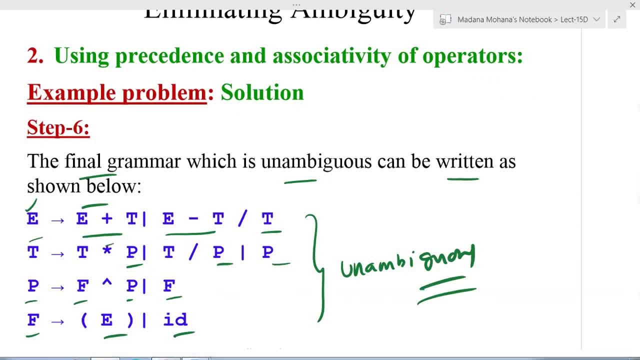 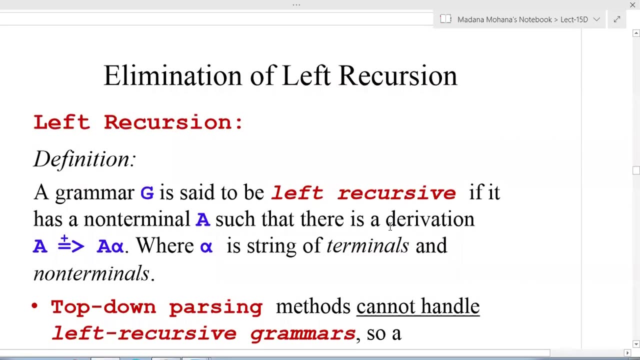 concept of precedence and associativity of operators for automatic type of grammars. these are the two methods for eliminating ambiguity. disambiguity rule under precedence and associativity of operators. so this is one transformation. now the second transformation: elimination of left recursion. this concept also little bit we discussed earlier in even formal language and automata. 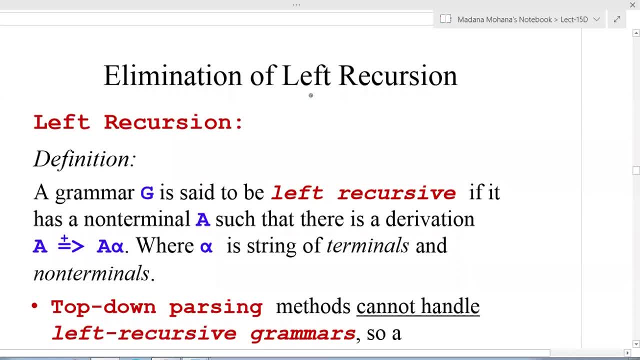 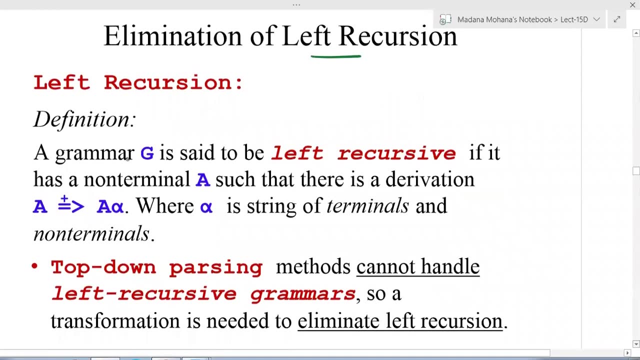 theory even in our previous lectures. now, how to eliminate that left recursion? why? because any grammar with left recursion that can't be used for top down parsing. that's why we have to eliminate left recursion. now, how to define a left recursion? let us see the definition. a grammar g is said to be. 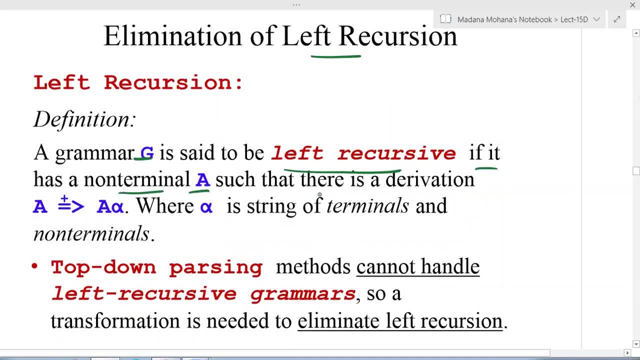 left recursive if it has a non-terminal capital, a, such that there is a derivation of the form. a derives a alpha. so here plus means with one or more steps of the derivation, substitutions are used. now here you can see: in this derivation the left hand side variable is same as the right hand. 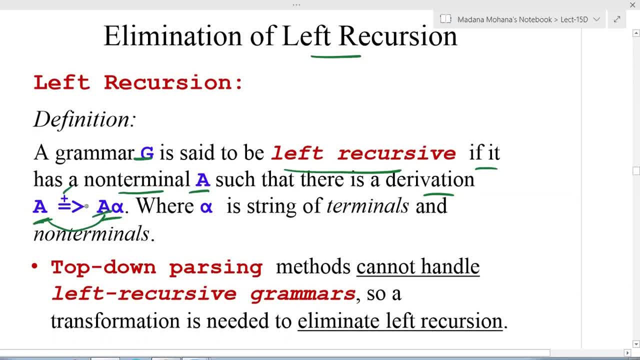 side, leftmost variable. so this is the form of left recursion where alpha is string of terminals and non-terminals. so if you can draw its derivation tree for a derives a alpha. now you can see a is the root, then a is substituted with a alpha. you can connect from left to right again a if you can. 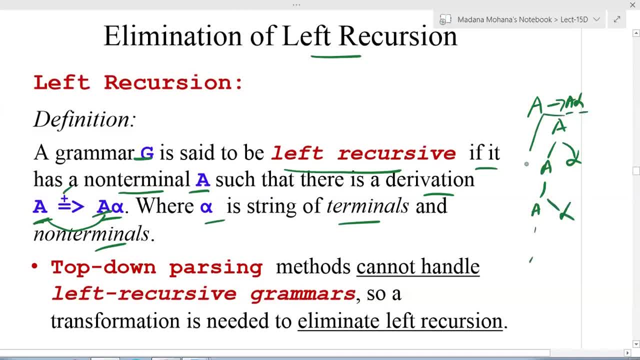 substitute a, derives alpha, and so on. this can be repeated. now this is called as left recursion. this is the general form of left recursion. you, that too. this is called as immediate left recursion. immediate means without any substitution itself, the given production itself in the form of left recursion. why? because the 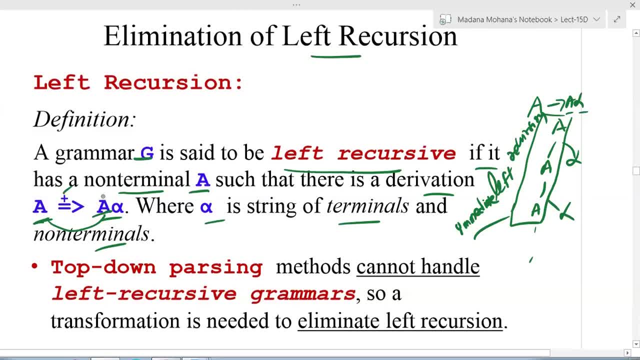 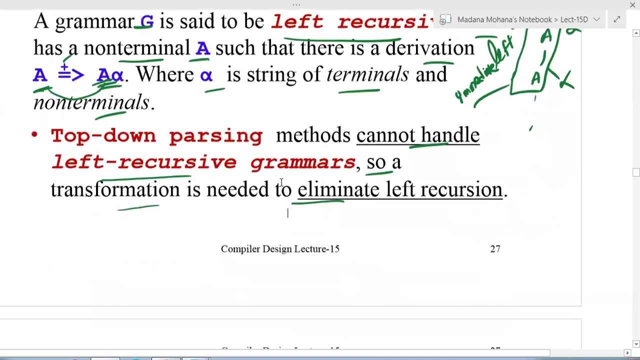 left hand side variable a is same as the right hand side of the production leftmost variable. that's why this is immediate left recursion. so top-down parsing methods cannot handle left recursive grammar, so transformation is needed to eliminate left recursion. so now on, this is a few examples- some this to you students- that we use in TriviaTrix: 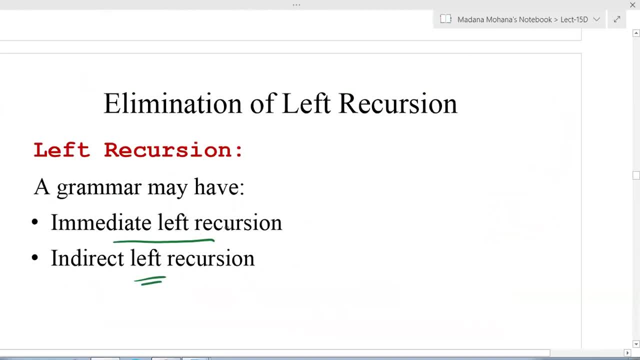 useful. I you got to kind of fancy it sometimes with alph� smart, your normal in training in the last class. you will haveuls elemental thing At that time. if you will get in the partial derivation, if you will get the left recursive form, then the grammar is said to be indirect left recursion. 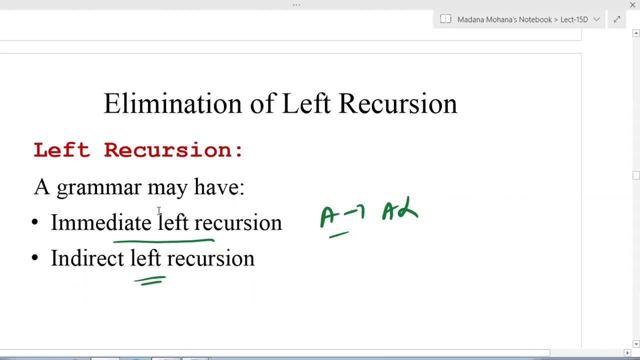 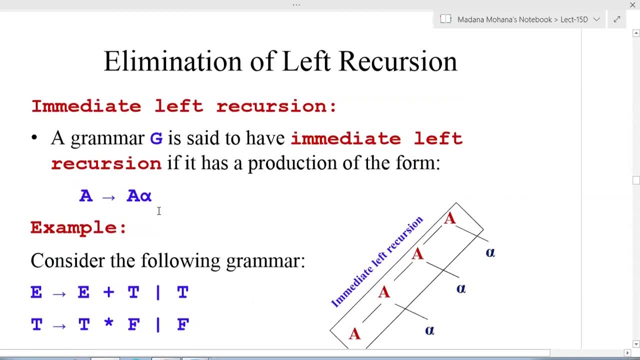 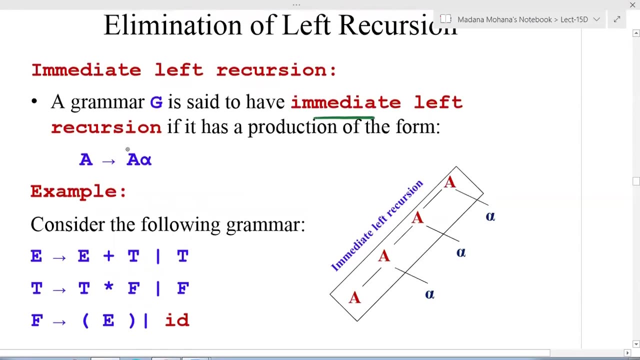 So the grammar may contains any of these, either immediate left recursion or indirect left recursion. We have to eliminate that left recursion. So now let us see immediate left recursion. just now, what we discussed, the same a grammar g is said to be have immediate left recursion if it has the productions of the form a derives. 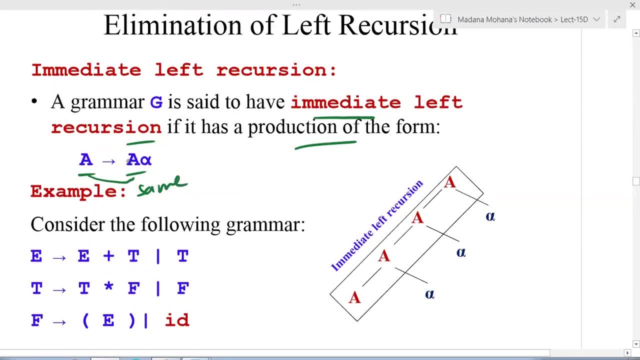 a alpha. So these two are same, left hand side variable and the right hand side, left most variable. So here you can see diagrammatically this can be represented: a derives a alpha, then again a derives a alpha. this is called as immediate left recursion. 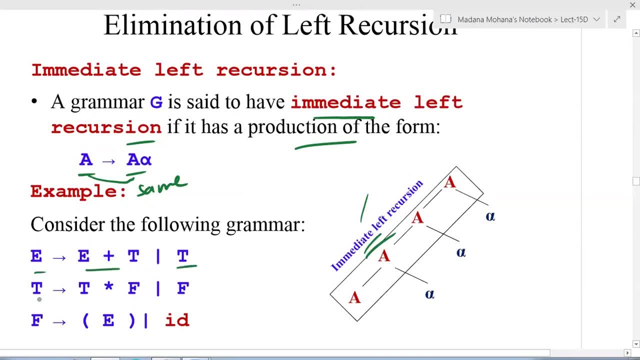 So let us consider one example: e derives e plus g or t. t derives t into f or f, f derives e within parentheses or id. In this grammar you can observe the first one: First production: e derives e plus t, So here these two are same, so which has immediate left recursion. then, second production: t derives. 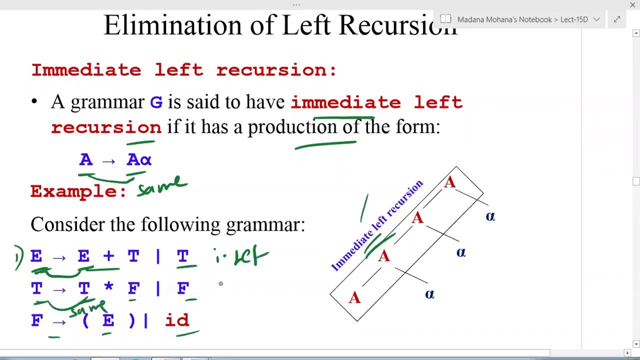 t into f. here also these two are same, so this grammar is also having immediate left recursion, whereas f derives e within parentheses or id. So it has no immediate left recursion because it start with left side left parentheses, So even it won't get indirect. also. 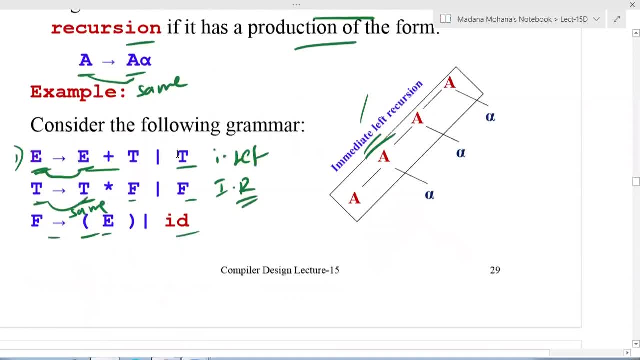 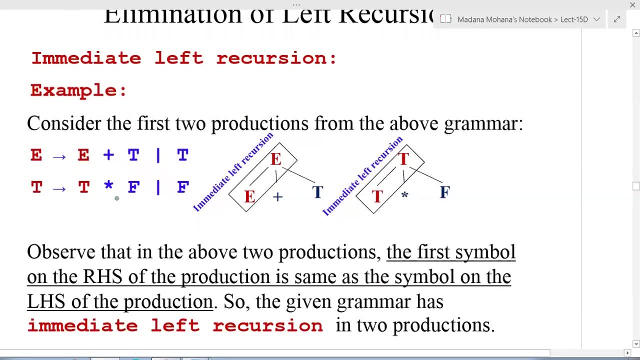 So let us consider this. So now this is example of immediate left recursion. So then, while constructing the derivation tree, are positive for these two productions. let us see diagrammatic representation: e derives e plus t, So here e now equivalents are e plus t. now these two are same, so which is called as immediate. 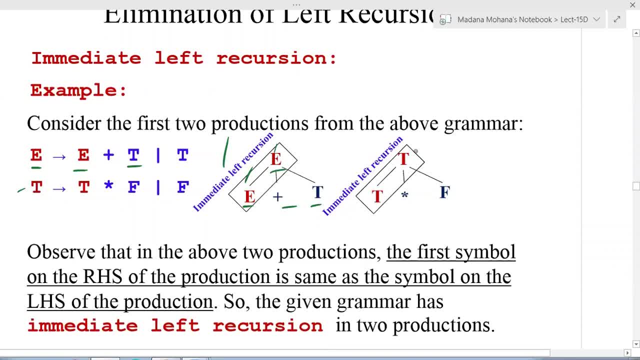 left recursion. then second production: t derives t into f, while drawing its tree, t derives t into f, So both trees are same. So immediate left recursion. observe that in the above two production the first symbol on the right hand side of the production is same as the symbol on the left hand side of. 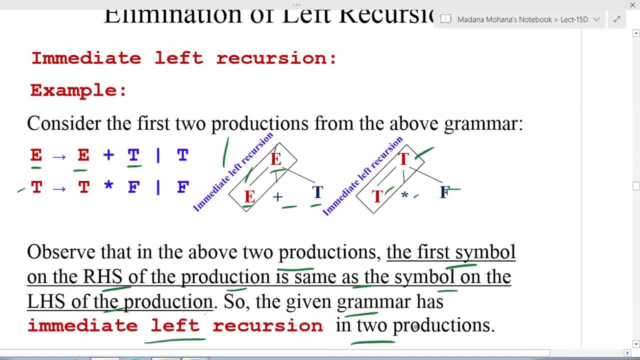 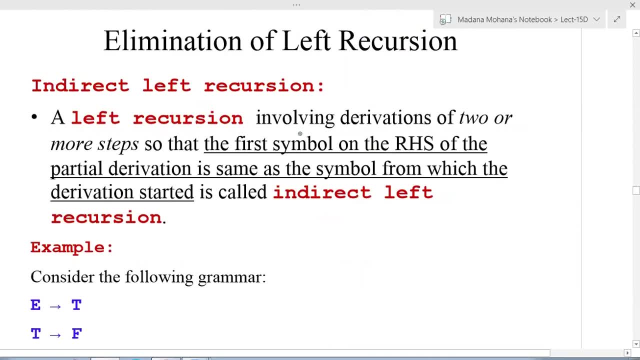 the production. So the given grammar has immediate left recursion in both productions. Now the second category: indirect left recursion: a left recursion involving derivations of two or more steps, so that the first symbol on the right hand side of the partial derivation is same as the second. 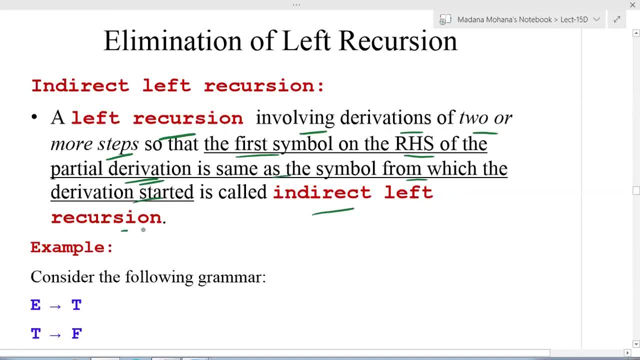 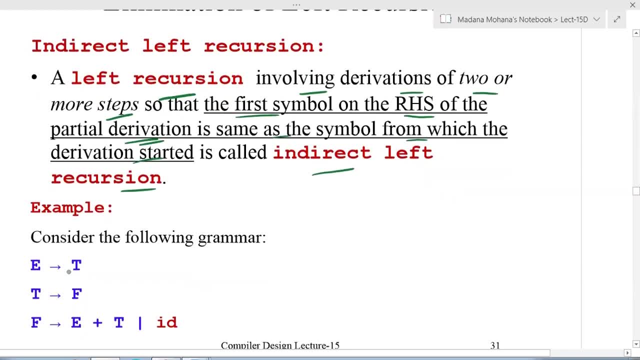 Now the second category. indirect left recursion is same as the symbol from which the derivation started is called as indirect left recursion what I explained previously. Now let us see the example. So consider the grammar: e derives t, t derives f, then f derives e plus t rd. 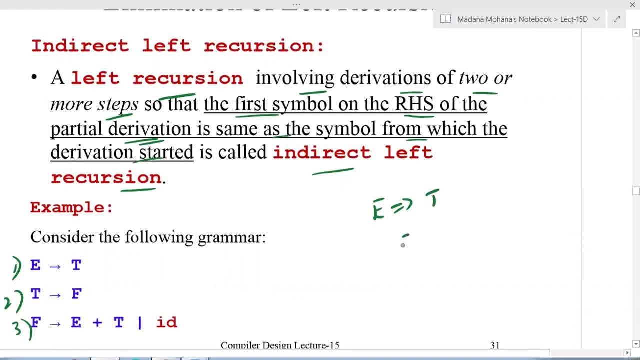 If you can do its derivation with starting symbol: e derives t, now what t contains. we have only f. now t derives f, then what f contains e plus t. Now, here you can see- this is step one derivation- Now what f contains e plus t. 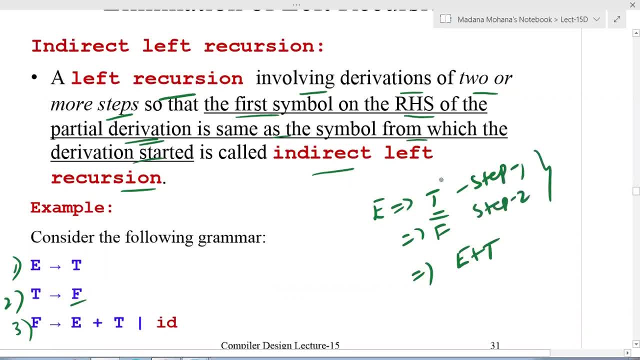 Now here you can see: this is step one derivation, Then this is step two derivation. So two or more steps. here two, two steps are used, then what we get here, e derives e plus t. Now here you can see: right hand side starting symbol is same as left hand side variable. 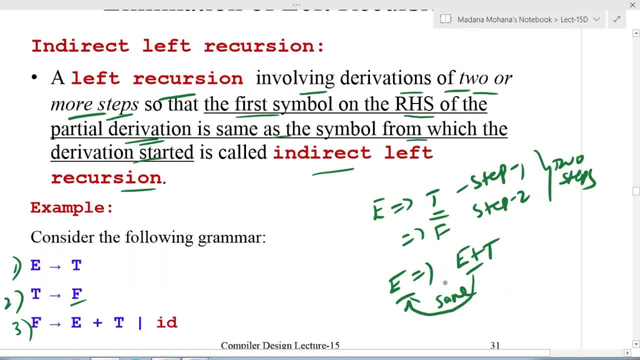 So here, after two steps, we got the left recursion. This is called as indirect left recursion, If any grammar consisting of indirect left recursion, This type of left recursion, that is indirect left recursion, That is indirect left recursion. So these two cases are there. 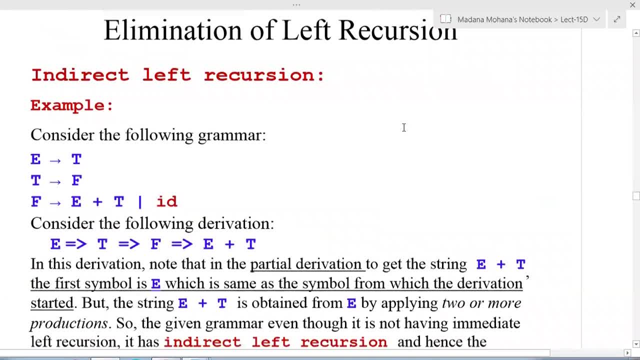 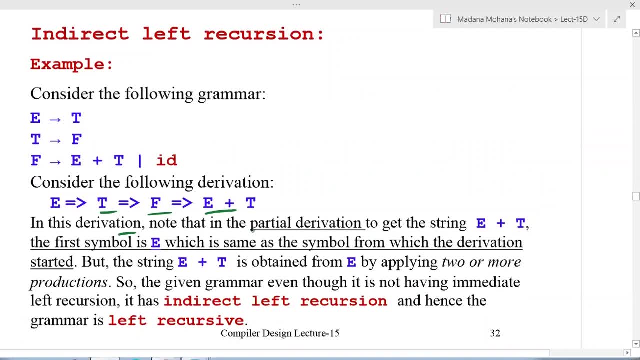 So now, here see what I explained. same thing is given here: e derives t, t derives f. f derives e plus t In this derivation. note that in the partial derivation to get the string e plus t, the first symbol is e, which is same as the symbol from the which derivation started, but the 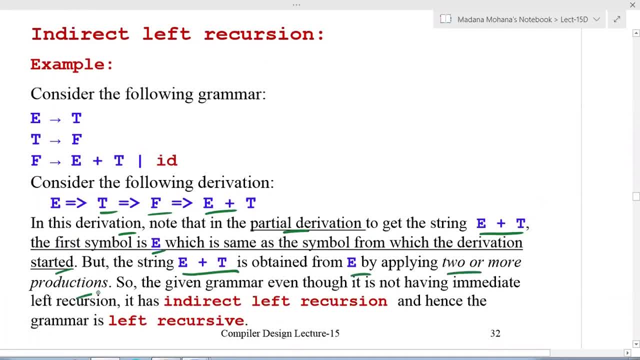 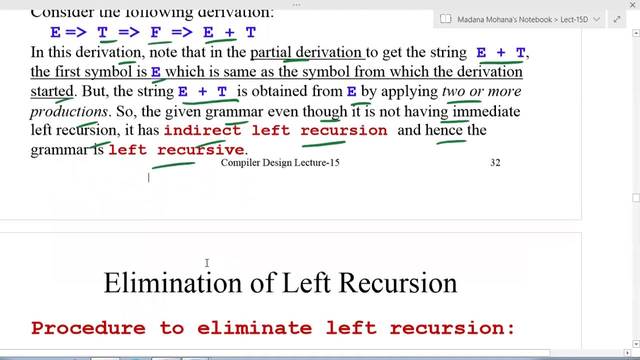 string e plus t is obtained from e by applying two or more productions. So the given grammar, even though it is not having immediate left recursion, but it has indirect left recursion, Hence the grammar is left recursive. Now how to eliminate left recursion? Here we have a simple procedure. Procedure to eliminate: 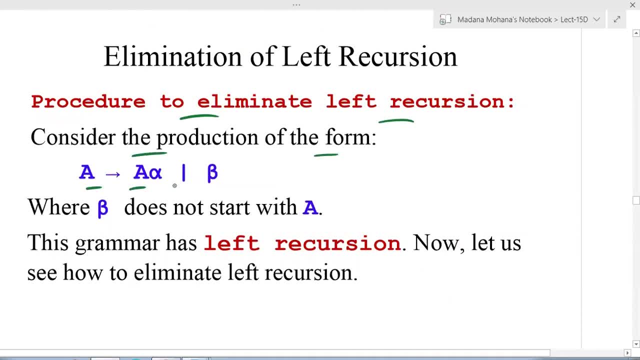 left recursion. Consider the production of the form a derives, a alpha or beta. You can consider only any one production in the right hand side which consisting of the same variable as in the left hand side variable, Then only that is in left recursive. Now here you can. 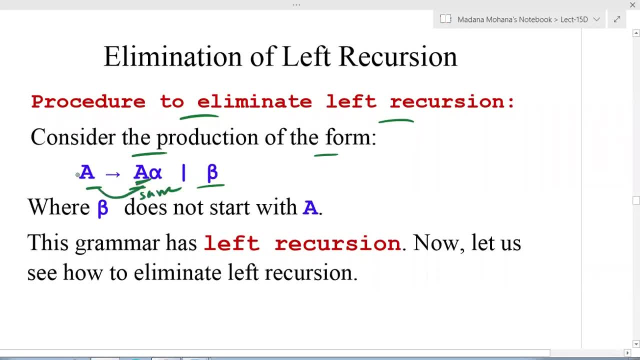 see. this is having left recursion. Right hand side a is same as left hand side variable a, where beta does not start with a. This is the condition. So then, this grammar has left recursion. Now let us see how to eliminate left recursion. 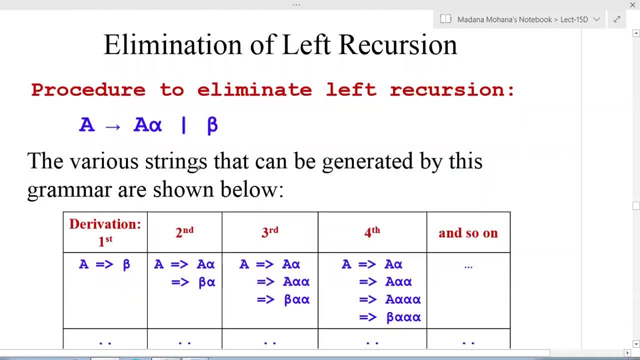 So first let us consider the following derivations for the given grammar a derives a alpha or beta. So here you can consider the derivations for this grammar: a derives a alpha or beta. Here you can see the first derivation. If you can substitute only beta, now you will. 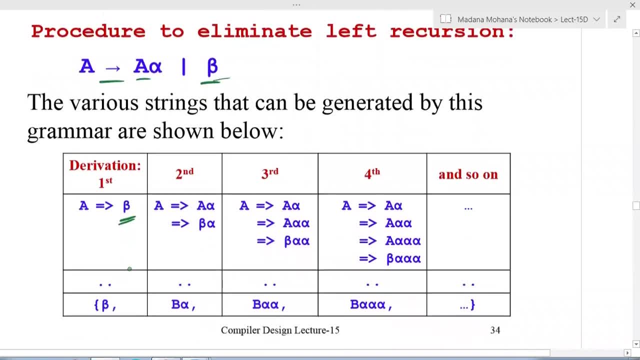 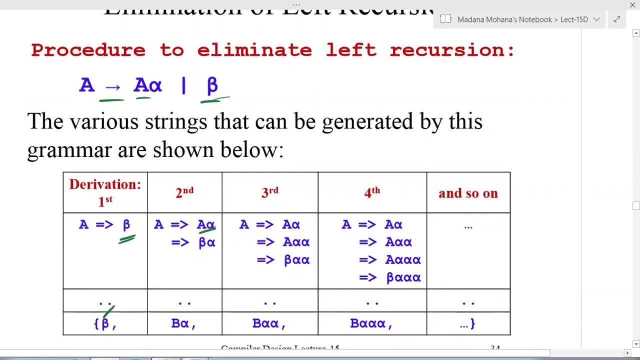 get a derives beta. Like: finally, here what you will get: a string starting with beta. only Second time, if you can take first production, a alpha. Again a is substituted with beta, with beta followed with alpha. here you will get. here you will get beta, alpha, then third, 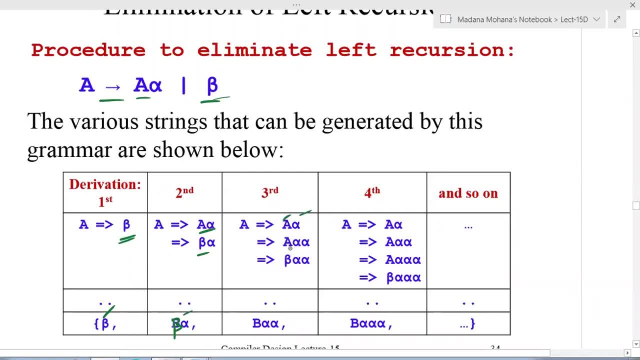 production again. you can take A alpha again. here you can substitute the same A alpha, then A is substituted with beta, then you will get beta alpha alpha. So here you will get the string beta alpha alpha. then fourth production: A ds A alpha again. A ds A alpha, alpha again. 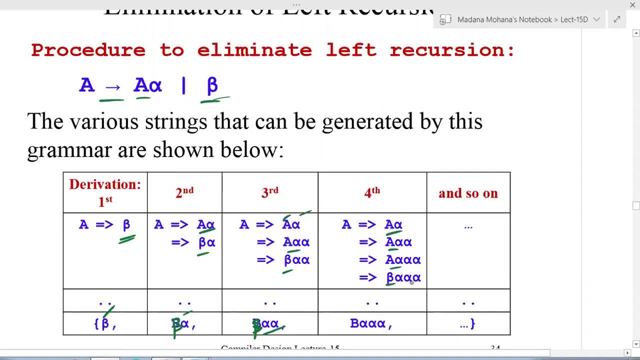 a dres, a alpha, alpha, alpha, then a is substituted with beta alpha alpha. So here you will get the production starting with the string beta, alpha, alpha, and so on. So now, here you can see. with this, you can observe every string starting with beta, followed by 0 or more alphas. 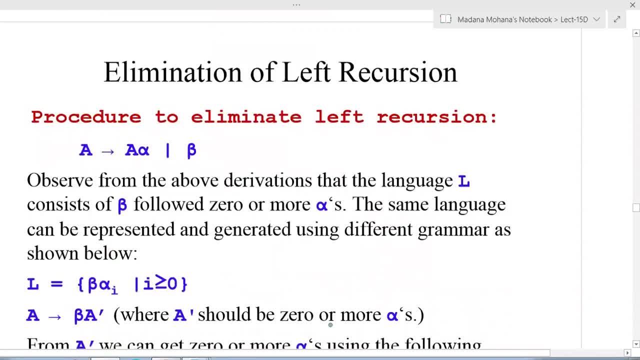 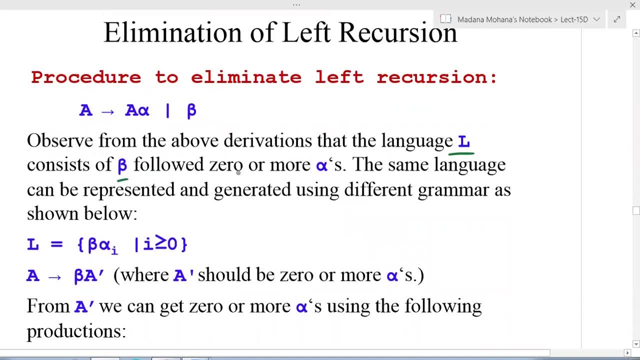 So now this can be written in the general form. let us see Observe from the above derivations that the language L consists of beta followed with 0 or more alphas. The same language can be represented and generated using different grammar, as shown below. Now the language. 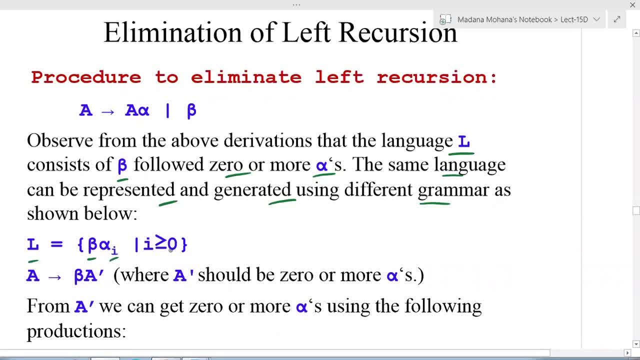 is L derives L equal to beta alpha. i where i greater than or equal to 0 means null. that is beta comma, beta, alpha, comma, beta alpha alpha, and so on. So this can be written as by the grammar: a derives beta by introducing a dash. 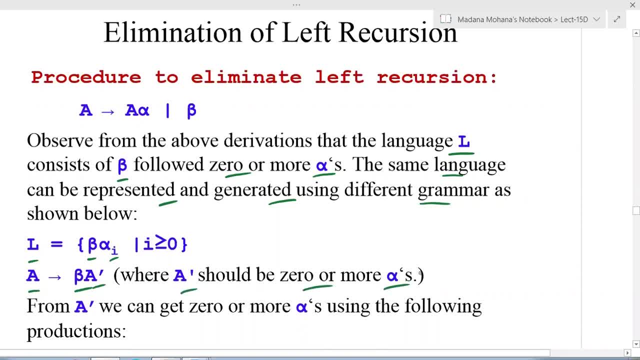 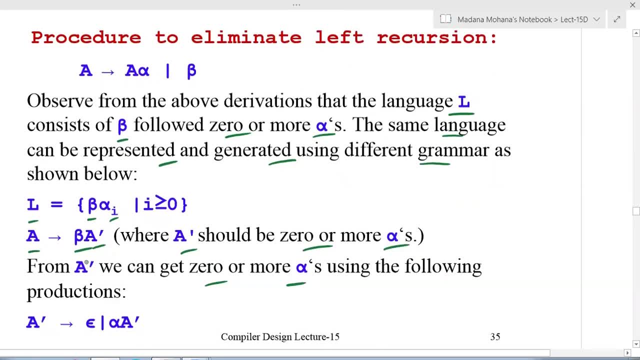 So where a dash derives beta, So now expect the function a dash denotes is the one that is set in the power g. So here the data should be 0 or more alphas. Now from a dash we can get 0 or more alphas. 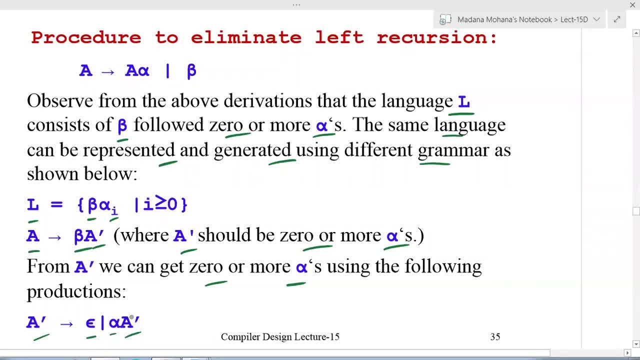 using the following production Now, a dash is the new. a dash derives null. that means zero or more alphas, alpha a dash. if you can substitute a dash as a null here, you will get alpha only. So like that now by using these two productions Here the first two. 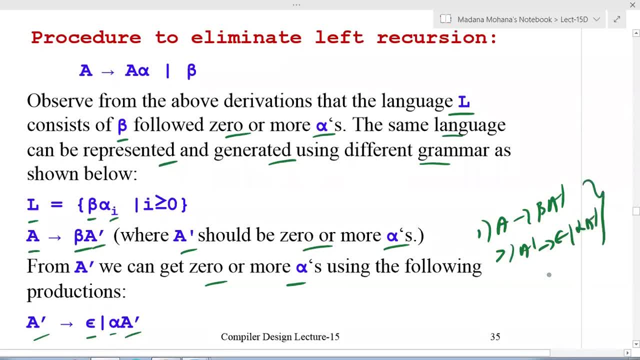 production: a derives beta a dash. Now, second production: a dash derives null alpha alpha. So if you use alpha only alpha, you get alpha only a dash, Because now we don't have alpha, So r alpha a dash. So now this is the equivalent grammar after eliminating left recursion. 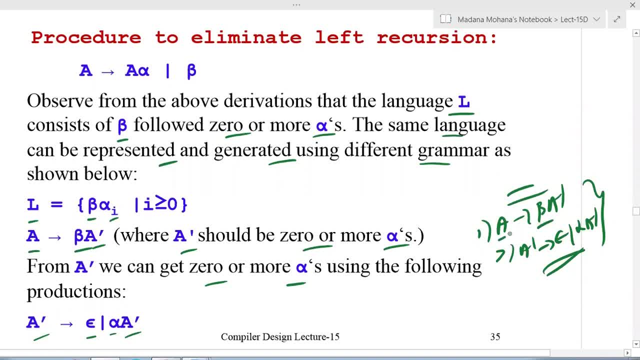 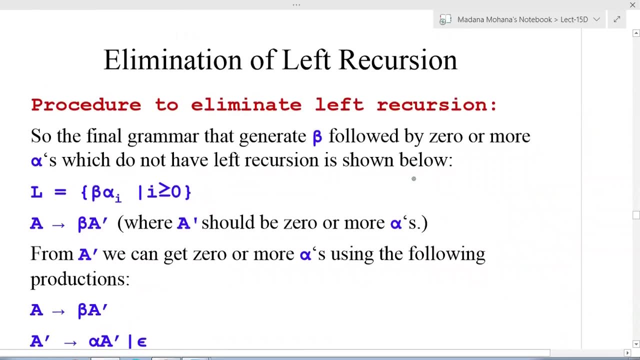 Now here you can observe in the right hand side, beta is not same as a. Then here a dash. also here you can see right hand side: it does not have the matching variable in the left side. So now the final grammar that generates beta, followed by 0 or more alphas which do not have left. 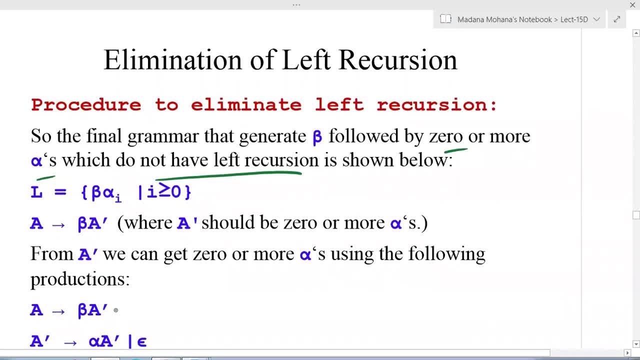 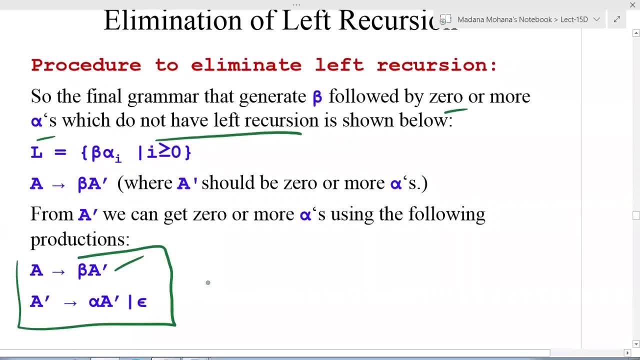 recursion is shown below. Here you can see a derives beta, a dash, then a dash derives alpha, a dash or null. This is the equivalent grammar after eliminating left recursion. This is called as non-left recursive grammar. So this we can use it as a rule or formula. So any grammar is in the 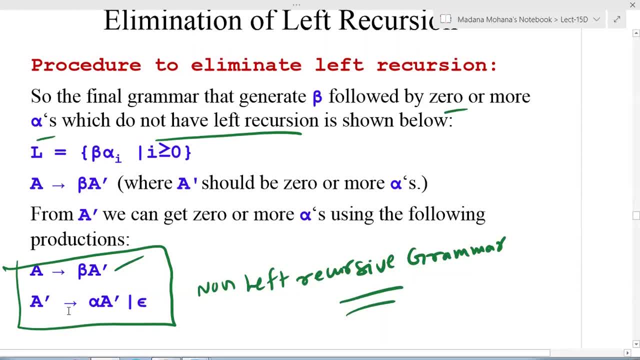 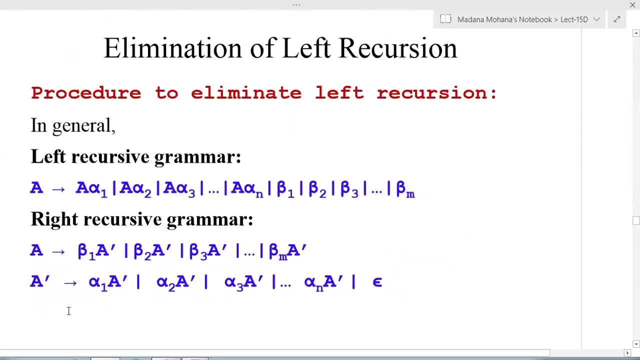 form of a derives, a alpha or beta. Now you can apply these two productions. then the grammar is in Non-left recursive. So now let us in general, if we have multiple productions starting with same variable as in left hand side variable, So a derives, a alpha 1 or a alpha 2 or a alpha 3. 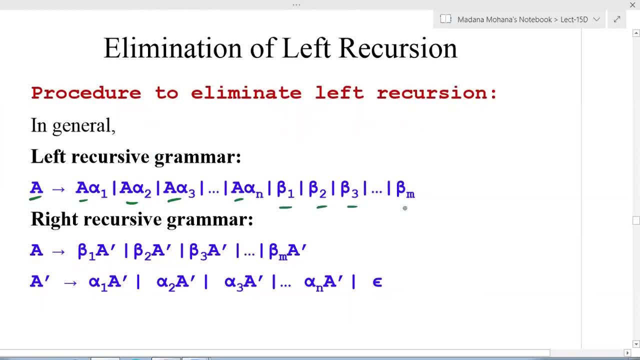 and so on. a alpha n or beta 1, or beta 2, or beta 3, and so on, beta m. So you have to consider only a's The variable, a matching with left hand side variable. So now, after applying the rule, if it has a derives, a alpha or beta. So now here: a derives beta, a dash rule 1.. Now, second rule: a dash. 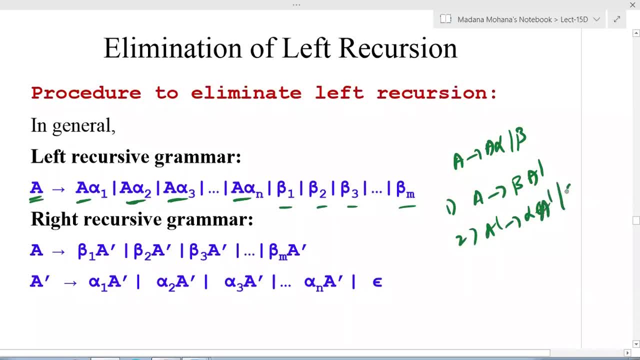 derives alpha, a dash or null. Apply this Now. first one is a derives beta a dash. Now here, a derives beta means n m betas are there. So beta 1 a dash, beta 2 a dash, beta 3 a dash, and so on. beta m a dash. 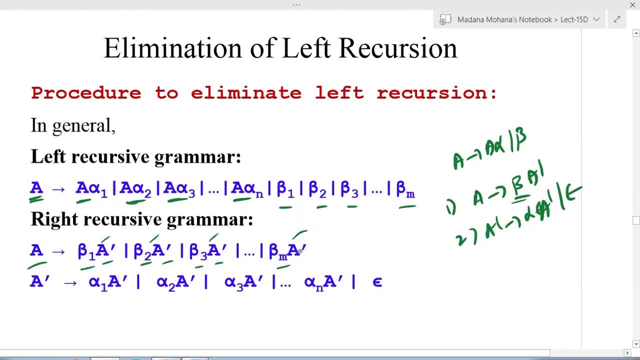 Here a dash is not changing, only beta values are changing. Now, what is a dash? here a dash derives alpha, a dash at last null. So alpha means here we have n alpha 1 to alpha, n alpha 1 a dash, alpha 2 a dash, alpha 3 a dash, and so on. alpha, n a dash or null. So for general productions this will consider. 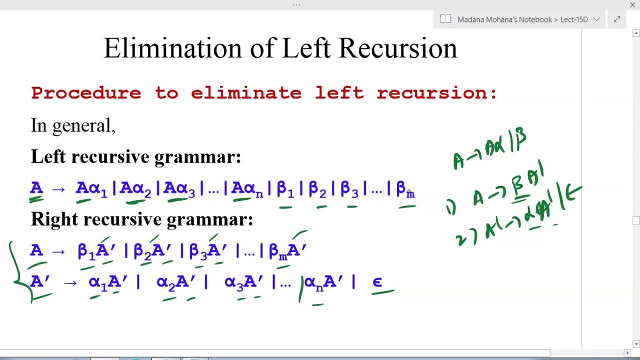 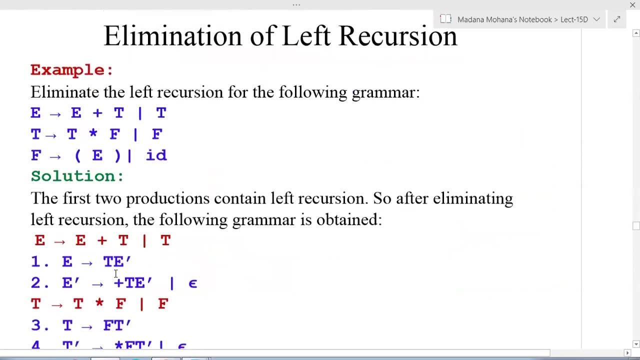 the general rule with n a productions and m beta productions. So by applying the same rules we can eliminate left recursion. Now let us demonstrate one example. So in examination you may get this type of questions also. Eliminate the left recursion for the following: 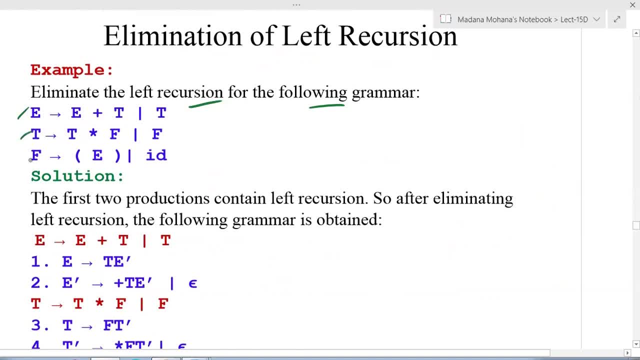 grammar. The grammar is: e derives e plus t, r, t, t derives t into f, r, f, f derives e. within parentheses already Same example. we explained. The first two production and the second production has immediate left recursion. The first two productions contain left recursion. So after eliminating left recursion, 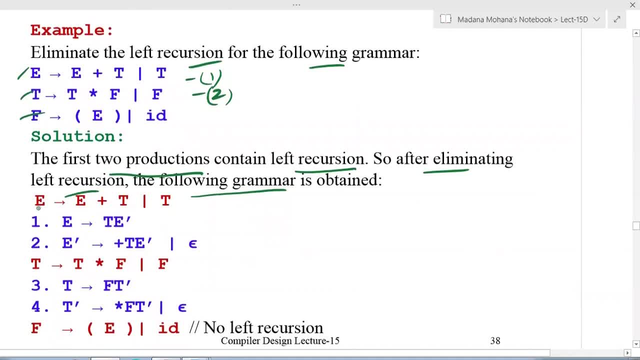 grammar is obtained. Now here you can see the first production. you can consider: a derives e derives e plus t, r, t. Now you can apply the general rule. It is in the form of a derives a. this is alpha, then r, beta. Now the first rule is a derives beta a dash. Second one is a dash derives alpha a dash. 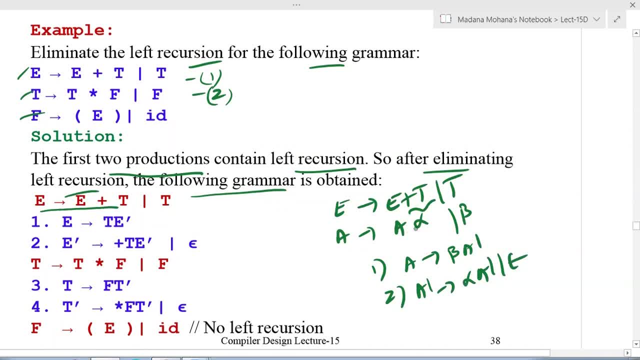 r null. Now substitute the a and r alpha and beta values here. So now a derives beta, a dash a means e e derives. beta is t Now e dash. Now e derives t e dash. Now a dash derives Here a dash means e dash Derives alpha. e is plus. 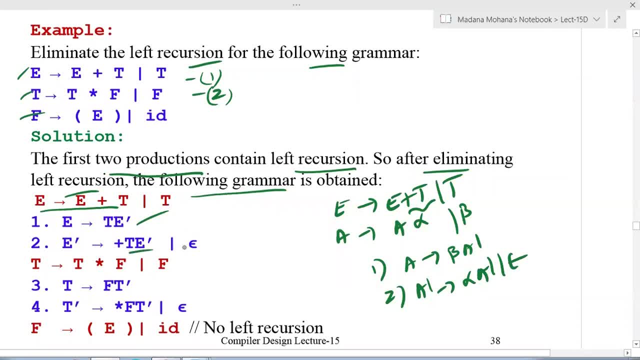 t Plus t e dash, So e dash derives plus t e dash, or epsilon or lambda. So this is the first production after eliminating left recursion. Same you can apply for second production: t derives f Now this is a. Now this is a. Alpha is star f. Now this is beta. Now the first rule is a derives. 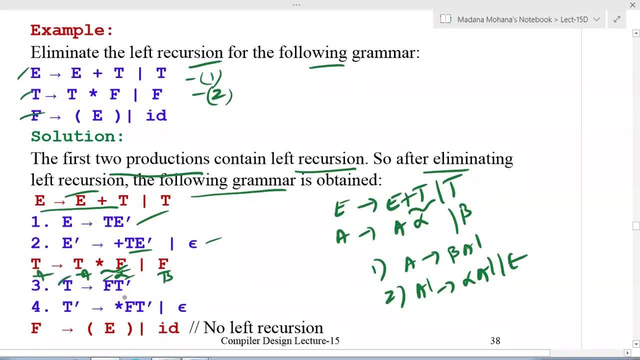 beta a dash. t derives f t dash. Now t dash derives alpha a dash. Alpha is star, f t dash or null. Now, finally, f derives e, within parenthesis: variety: No left recursion. Therefore, this is the equivalent grammar after eliminating left recursion. This is very simple, Simply applying the two production. 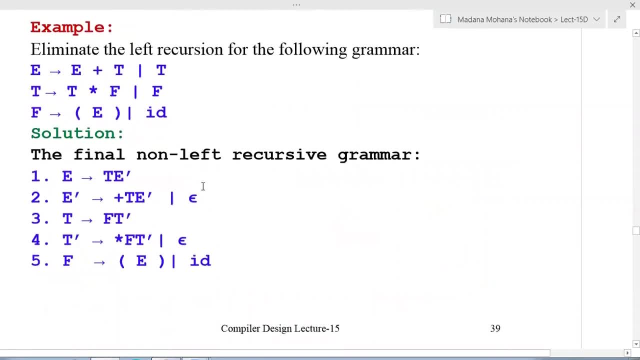 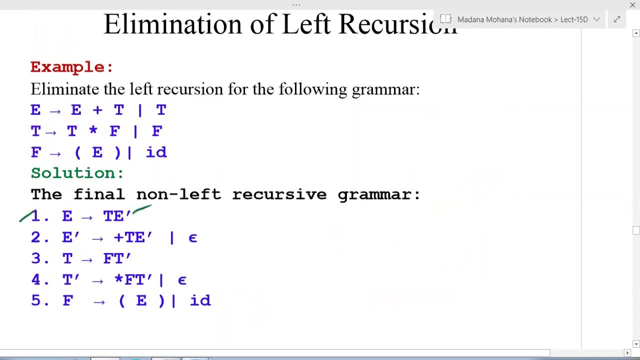 rules which are in non-left recursive. The final non-left recursive grammar is: You can write all the production starting with starting variable. First one, e derives t, dash, Then here e dash derives plus t, dash or null, Then t derives f, t dash, Then t dash derives star, f, t, dash or null, Then f derives e within parenthesis variety. 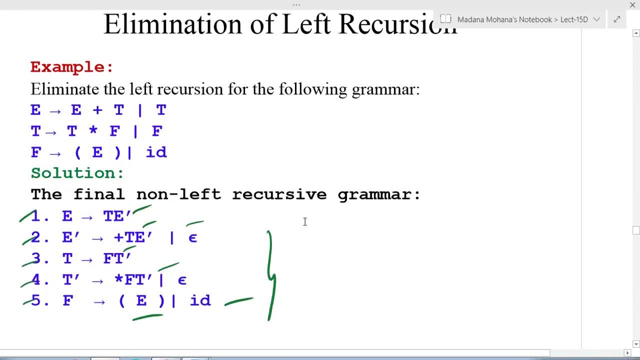 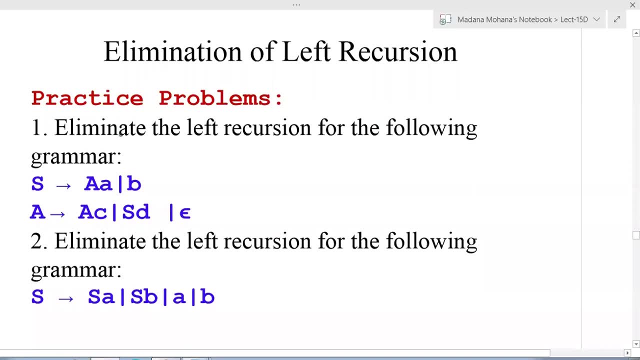 So this is the final grammar which is in non-left recursive form. So like that you have to eliminate left recursion. So now, here some practice problems are given. You have to practice Eliminate left recursion for the following grammar. Here you can see s derives a, a or b. So here no left recursion. 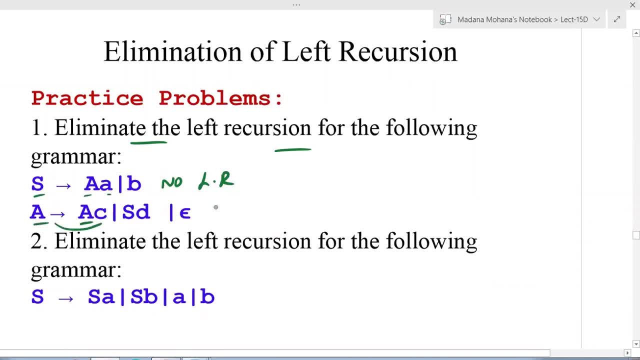 Here you can see: a derives a, c. Here it has contains left recursion. Contains left recursion. So you have to eliminate, Apply the rule. Then, second example: s derives s, a or s b or a or b. Here you can see: both are same with this one, So it is left recursion. 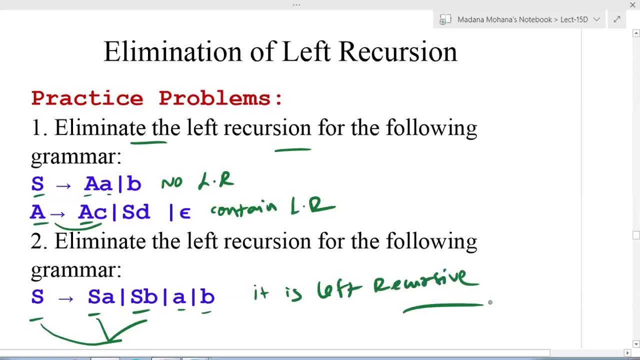 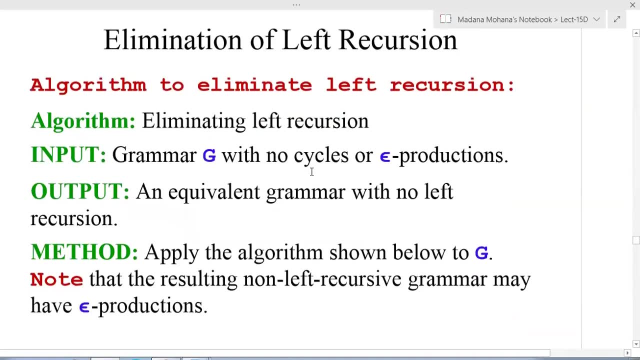 So you have to eliminate left recursion using the two rules. what we discussed. Then, coming to algorithm for eliminating left recursion, Whatever the process, we used Same thing in the form of algorithm. The algorithm name is eliminating left recursion. The input is this algorithm, a grammar. 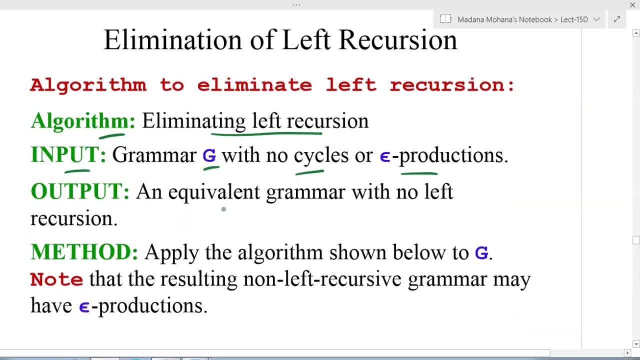 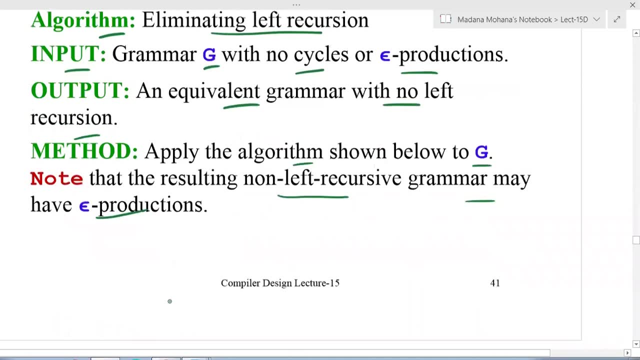 g with no cycles or epsilon production, Output is an equivalent grammar with no left recursion. Then method: Apply the algorithm shown Below to g. Note that the resulting non-left recursive grammar may contains epsilon productions also, That is, after eliminating left recursion. Now the method is the same. what we 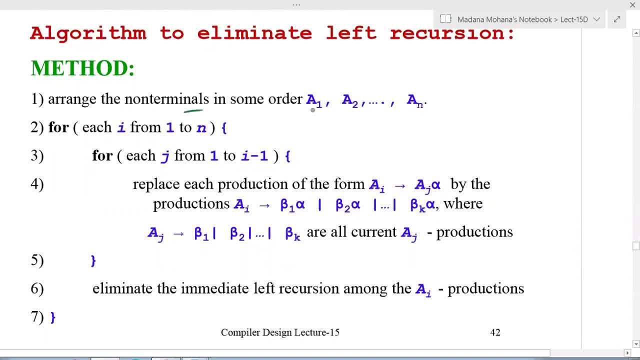 discussed in example. Arrange the non-terminals in some order, like a 1, a 2 and so on. a n For each i from 1 to n, Then for each j from 1 to i minus 1.. Replace each production of the form a i derives. 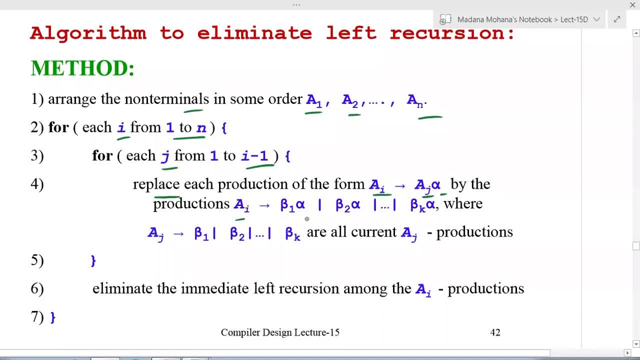 a j gamma by the production of a j gamma. So you have to eliminate left recursion. Now the method a j is given in this form: For any ah j productions: a? i derives beta 1 alpha or beta 2 alpha, and so on Beta, k, alpha. where a? j derives beta 1 or beta 2 and so on: Beta. 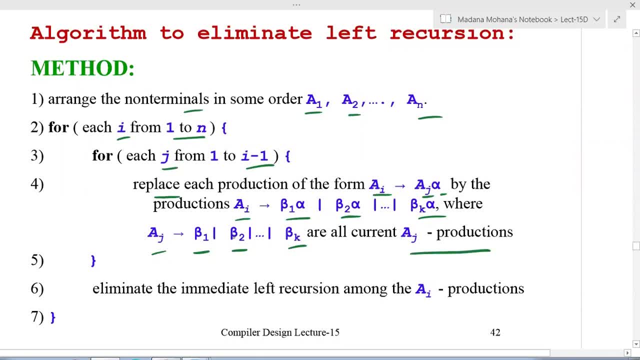 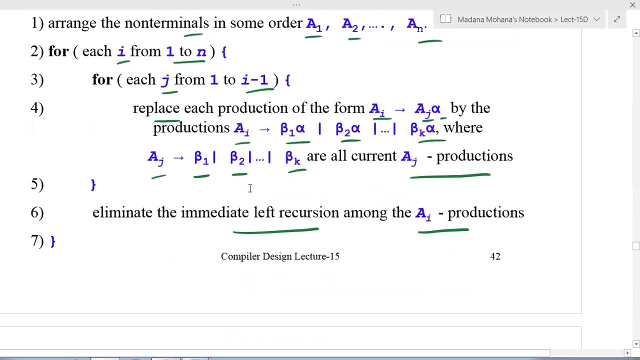 k, all are current a, j productions. Now, whenever the productions are transferred in this form, then we have to eliminate immediate left recursion among a- i productions. So the same example, whatever the method we applied, Same is given in this algorithm. So then, coming to next concept, Left. 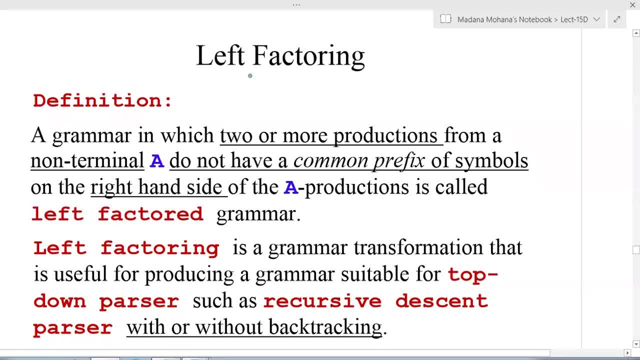 function Ah j of the worked ant. You have to eliminate the non-determined courage of left factoring, so this is also another important one. so you have to apply any grammar before applying to top-down parsing. so the definition of left factoring: a grammar in which two or more productions. 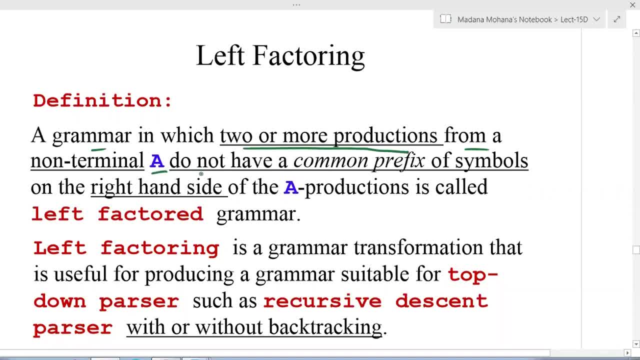 from a non-terminal capital, a, do not have, do not have a common prefix of symbols on the right-hand side of the air productions. this is called as left factored grammar. suppose, if you have a derives a derives alpha 1 beta or alpha 1 gamma. now, here you can see two or more productions starting with. 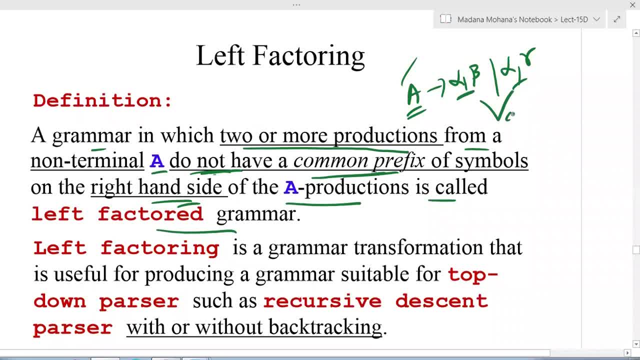 one variable, so having common prefix. now here you can see this is common prefix. so this is not exist in a grammar, then the grammar is said to be left factored grammar. so if any of this situation occurred, then you have to apply left factored grammar. so if any of this situation occurred, then you have to apply left factored. 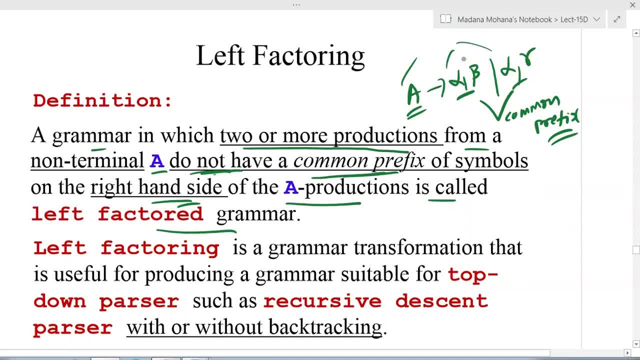 concept, then this can be factored out by taking common prefixes out. so that is the concept of left factoring. so left factoring is a grammar transformation that is useful for producing a grammar suitable for top-down parsers, such as recursive descent parser, with or without back. 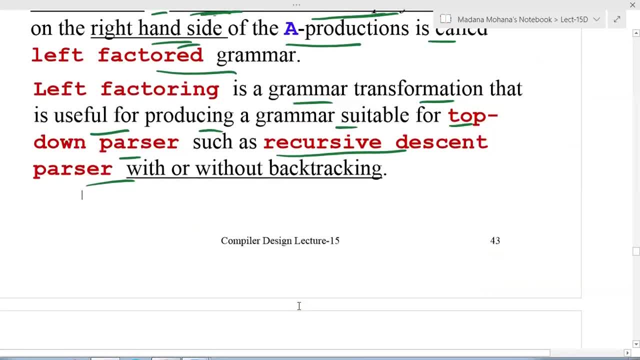 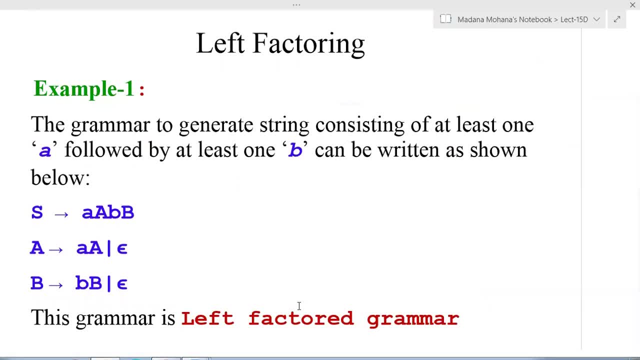 this is one of the first technique of top-down parsing. so now let us consider one example, the grammar to generate a string consisting of at least one symbol a, followed by at least one b, can be written as shown below: s derives a- terminal a- variable a- terminal b- variable b. now a derives terminal a- variable a. 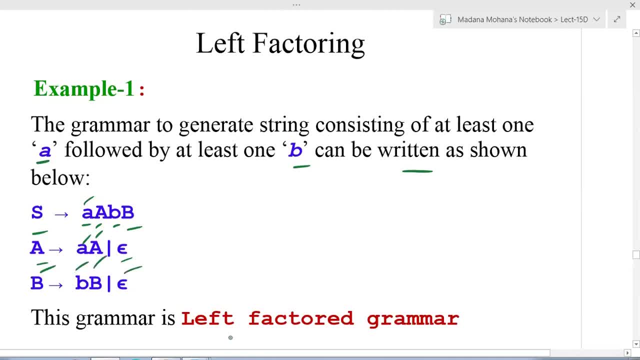 ornale v derives terminal b, variable b, ornale. this grammar is left factored grammar. the reason here: you can see. so here for a. for a contains two productions, starting with terminal a, ornale. so no two common prefixes and s are one production. oh, so you can see. the s has only one production, so we can't consider this one. Then b contains two productions. 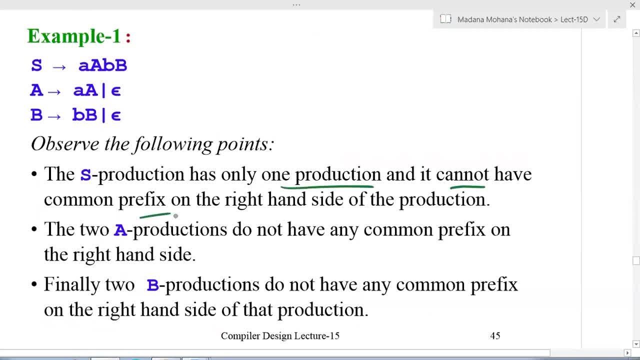 So it has no two common prefixes. therefore this grammar is left-factored grammar. so now here the same observations given here: the s production has only one production and it cannot have common prefix on the right hand side of the production that two a productions do not have. 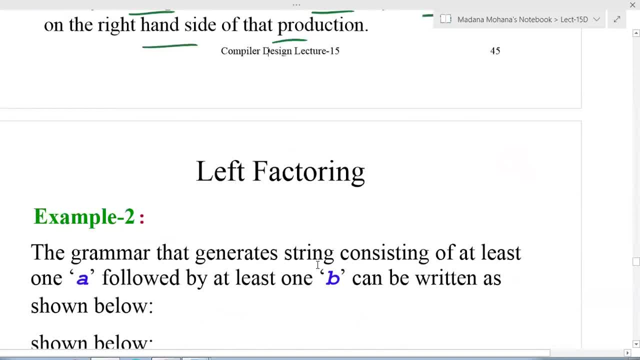 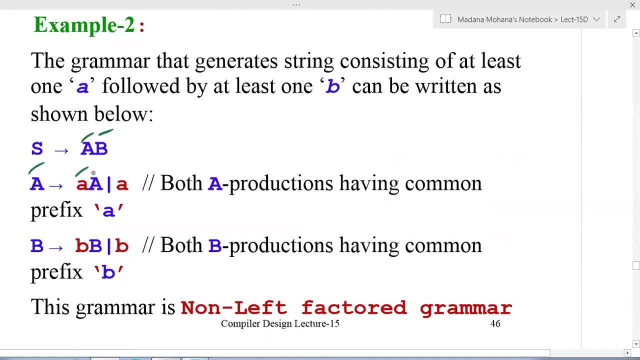 production. therefore this is left factor grammar. then another example. let us see s derives capital, a, capital b. now a derives terminal a, variable a or terminal a. here you can see both a productions having common prefix a, highlighted in red color. here you can see two productions, so having common prefix, starting with same terminal a. then b derives terminal. 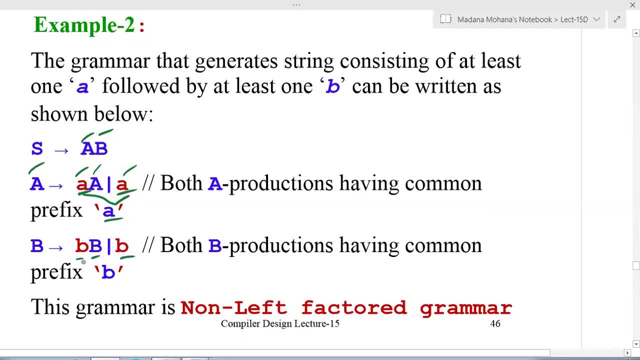 b, variable b or terminal b, here also both b productions having common prefix, that is b. so therefore this grammar is non left factored grammar, for this type of grammar are not used for top down parsers, so we have to apply the concept of left factoring. then you have to. 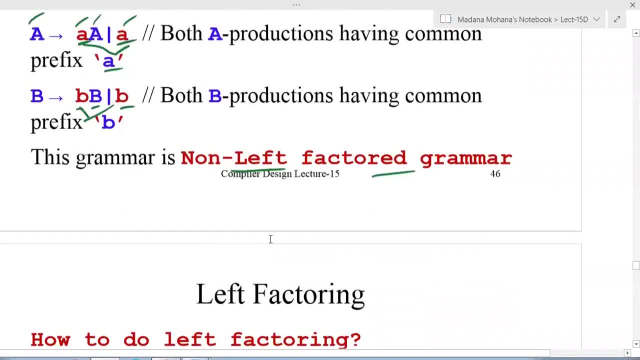 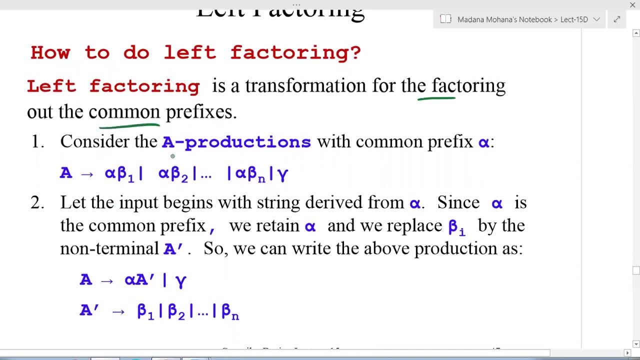 factoring out the common prefixes, but then how to do left factoring. so left factoring is a transformation for the factoring out the common prefixes. consider the a productions with common prefix alpha as the general form. a derives alpha beta or alpha beta 2, and so. 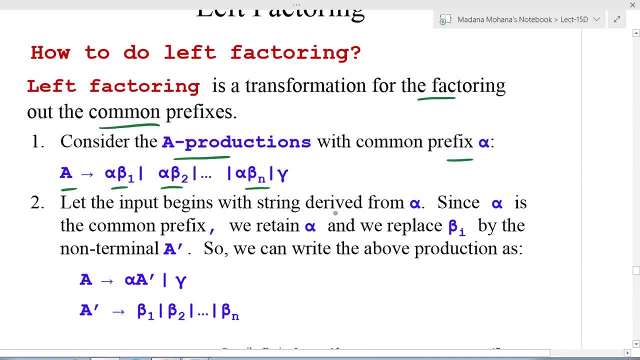 on alpha, beta, n or gamma. so let the input begins with the string derived from alpha. since alpha is the common prefix, we retain alpha and we replace beta i by the non-terminal a dash, so we can write the above productions as now. here you can see: a derives, alpha remains safe. 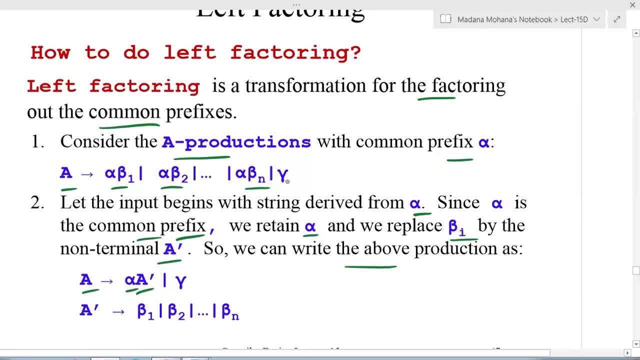 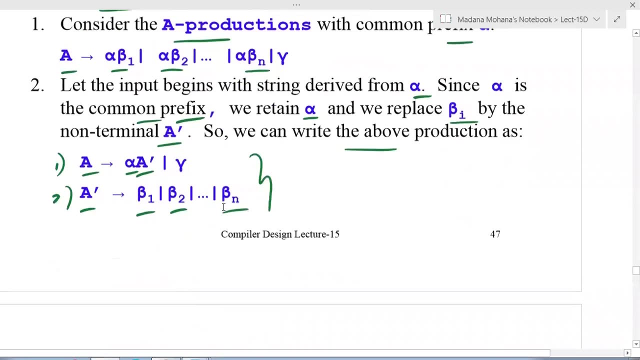 all beta values are replaced with a dash or gamma, remains safe. now, this is the rule one, then rule two. now, what is a dash? a dash derives all beta values, beta one or beta two, and so on, beta n. so these two rules are used for applying left factoring for any grammar. now let us 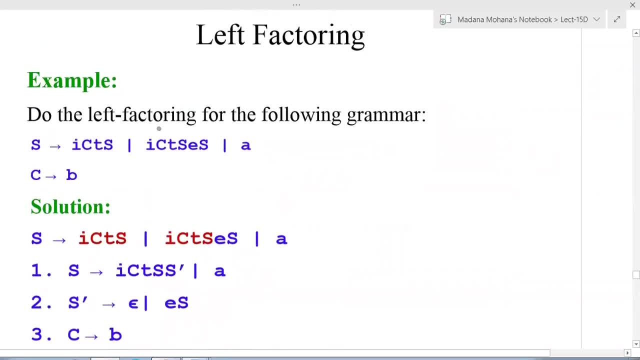 consider one example. so here do the left factoring for the following grammar: yes, there is i c t s, i c t s, r a c there has to be. here you can see i c t s, first production, second production, i c t s. so up to this. here you can see having common prefix. these two are same. 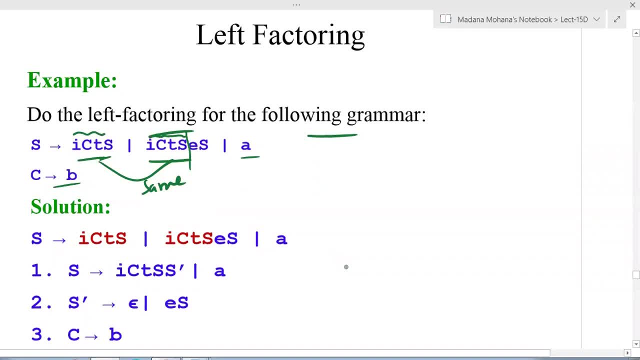 so therefore this is a non left to factor grammar. we have to apply left factoring, so by applying the general rule. so now s derives i c t s or i c t s, es or a. the highlighted color i c t s is common prefix in both of s production, so then you can take this i c t s as it is. 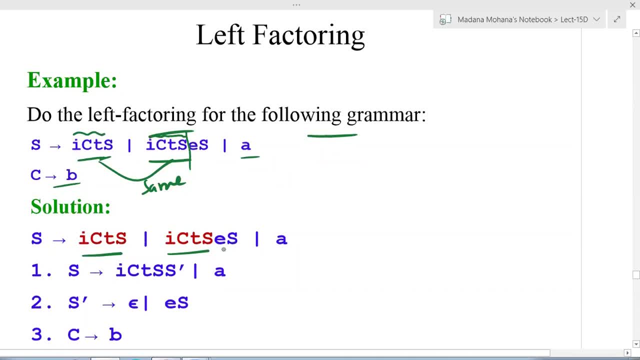 then remaining beta values. you can substitute using s dash. so here s dash is introduced now remains same the alpha s dash, the terminal a, gamma also remains same. this is gamma. now. what is s dash here here? null is there now here? yes, so s dash dash epsilon. or yes, then c dash b. 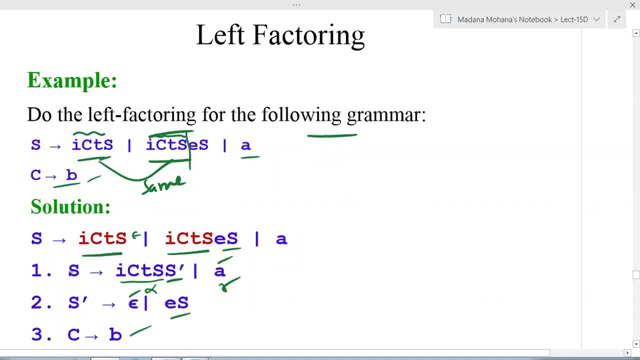 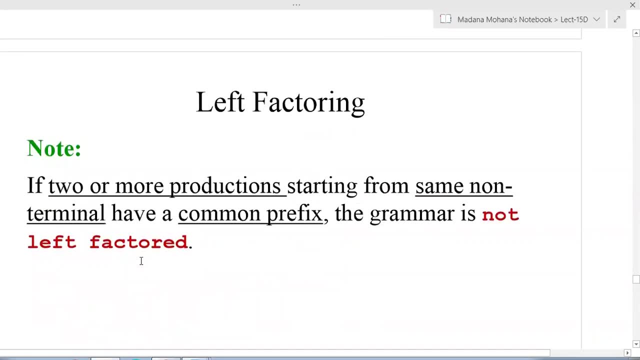 this is already left factor grammar, so we no need to apply now. this is the equivalent grammar after applying left factor grammar. so now let us see one important note: if two or more productions starting from same non-terminal have a common prefix, suppose two or more production, suppose. 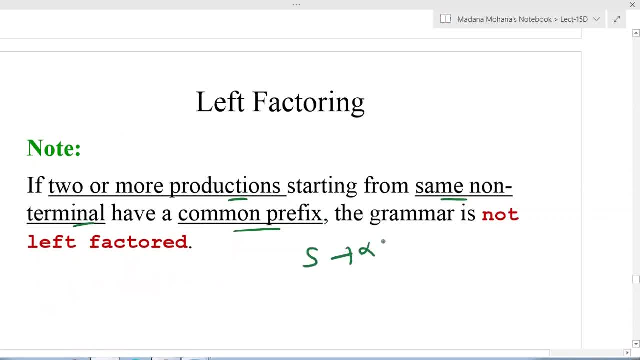 starting with the same non-terminal: s derives alpha a, now s derives alpha b. here you can see two or more productions starting from same non-terminal: see same non-terminal having common prefix here. so even this grammar is not left factor. why? because whenever you can combine these two, alpha a or alpha b, 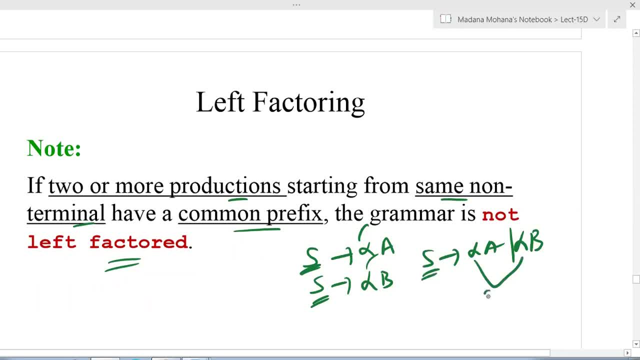 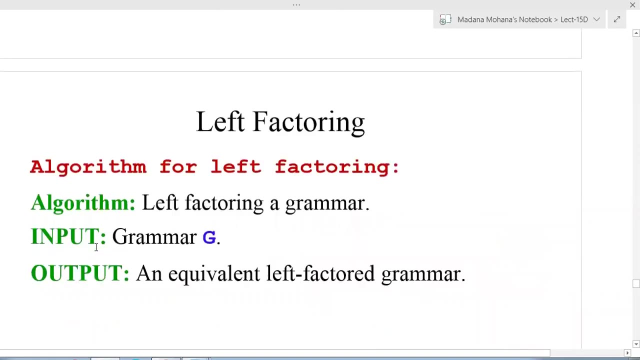 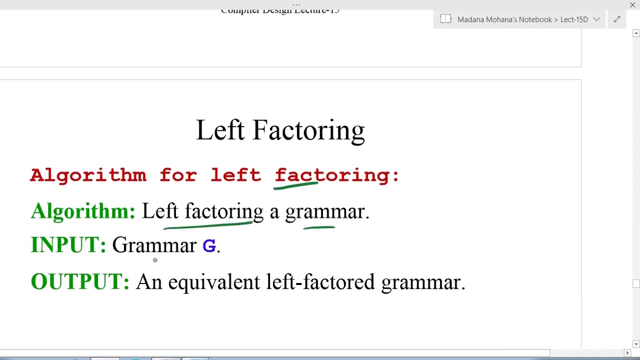 why? because starting with same non-terminal, so here common prefix is there. so therefore this is not left factor grammar, this is non-left factor grammar. for this also you have to apply left factory. now let us see the algorithm: same. whatever we explain the algorithm for this algorithm for left factory, the name is left factor a grammar, input is a grammar g. 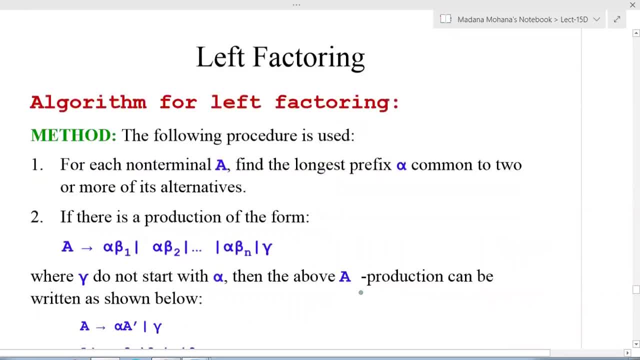 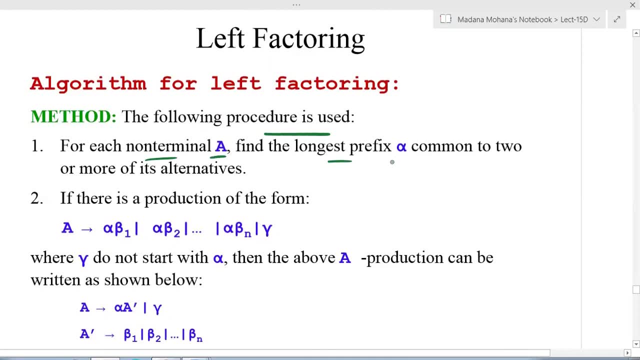 output an equivalent left factor grammar. now let us see the method. the following procedure is used for each non terminally: find the longest prefix alpha common to two or more of its alternatives. if there is a production of the form what we discussed, a del s alpha beta one or alpha beta two, and. 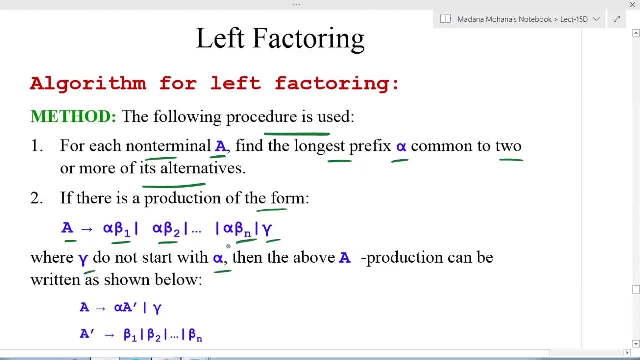 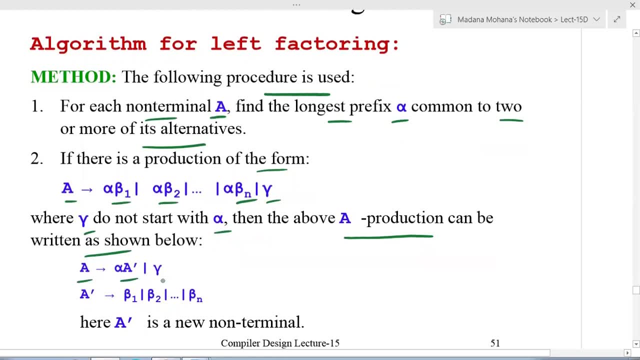 so on alpha, beta, n or gamma. where gamma do not start with alpha, then the above a productions can be written as shown below the two rules, what we discussed here, del s alpha, a dash or gamma. then a dash alpha is mentioned as alpha for all, b, G, where this summation is E to the 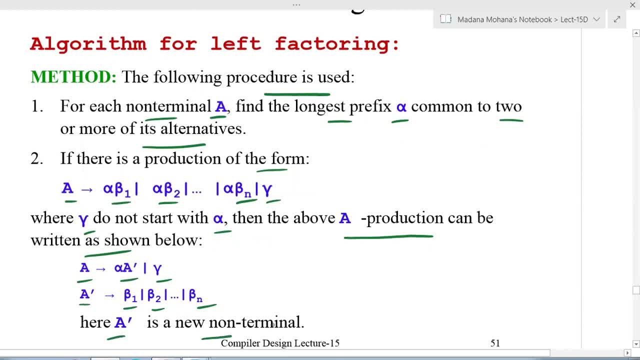 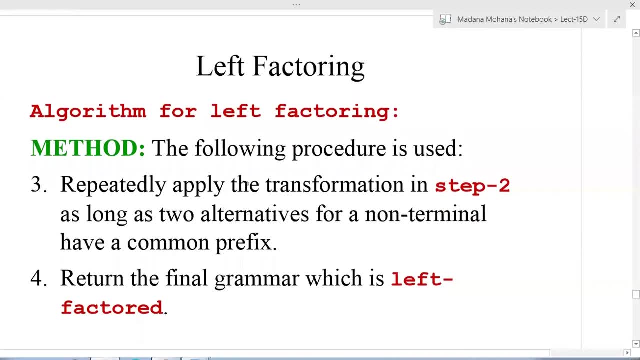 data. there is beta 1 or beta 2 and so on. beta n, where a dash is a new non-terminal. So this is the algorithm. Now repeatedly apply the transformation in step 2 as long as two alternatives for a non-terminal have a common prefix. Return the final grammar which is left-factor grammar. 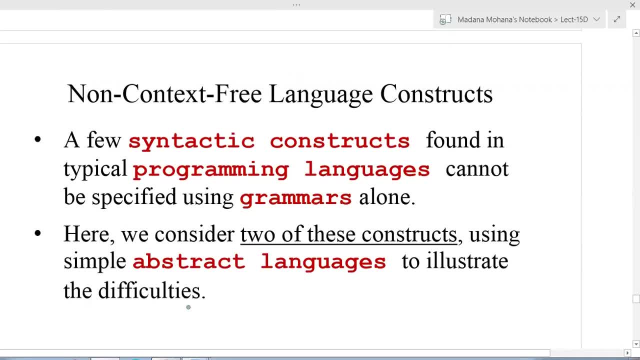 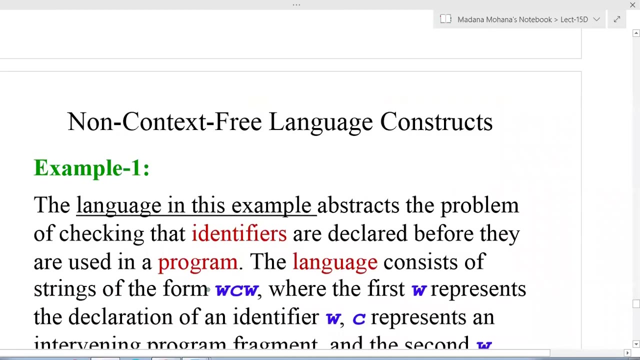 Now the last concept: non-contextual language constructs. That means non-CFL. So a few syntactic constructs found in typical programming languages cannot be specified using grammar alone. Here we consider two of these constructs using simple abstract languages. to illustrate the difficulties, The first example: let us see The language in this example abstracts the. 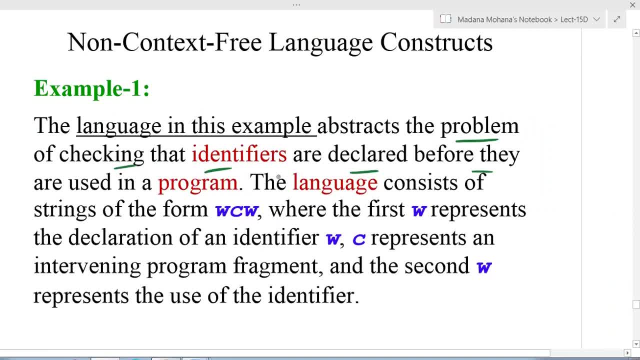 problem of checking That identifiers are declared before they are used in the program. The language consists of the strings of the form WCW, where the first W represents the declaration of an identifier W, Then C represents an intervening program fragment and the second W represents the use of the. 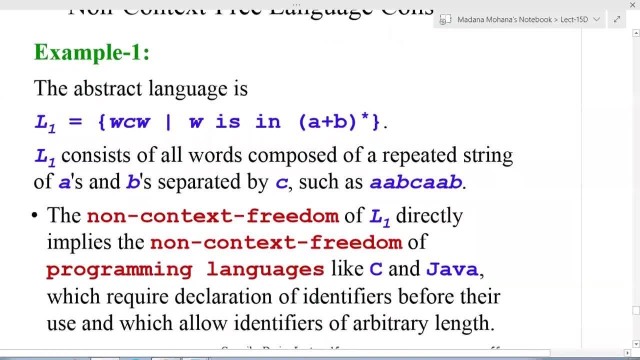 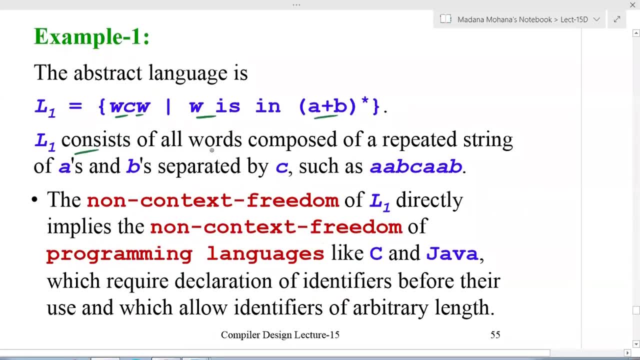 identifier WCW. So this is the example of palindrome string language. Now the language is L1, equal to WCW, where W is an A plus V, whole closure. Here L1 consists of all strings or roots composed of A repeated string of A's and B's separated with C, such as AAB, C, AAB separated with C. 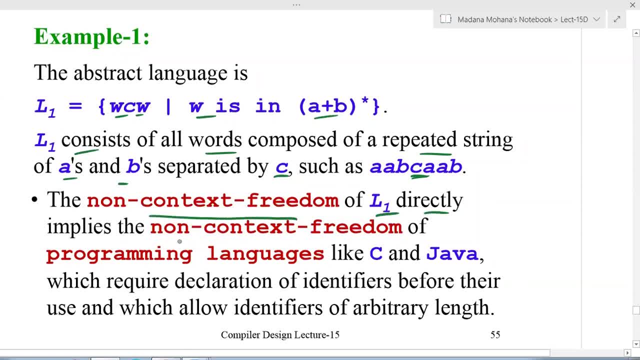 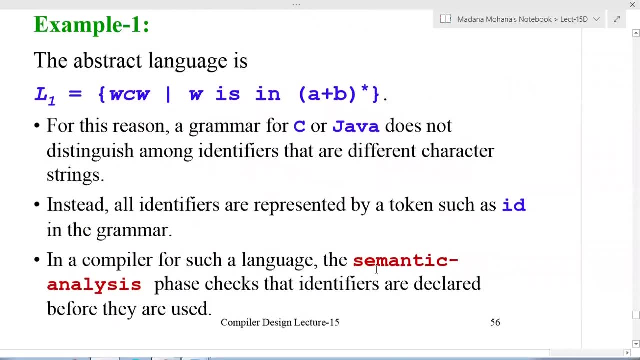 The non-context freedom of L1 directly implies the non-context freedom of programming language like C and Java, which require declaration of identifiers before their use and which allow identifiers for any arbitrary length. This is one non-contextual language. So now, for this reason, a grammar for C or Java. 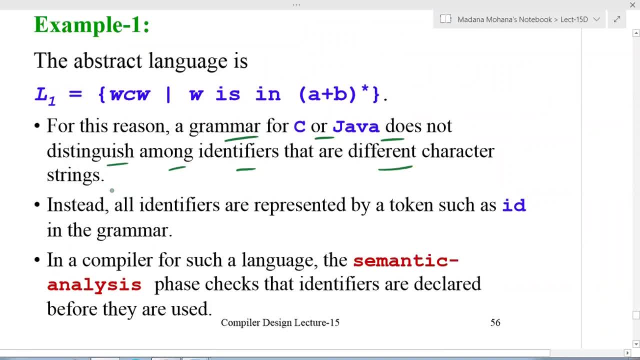 does not distinguish among identifiers that are different characteristics. Instead, all identifiers are represented by a token, such as ID, in the grammar. In a compiler for such a language, the semantic analysis phase, which is the third phase of compiler, takes that identifiers which are declared before they are used. So this is the one example for considering non-contextual language. 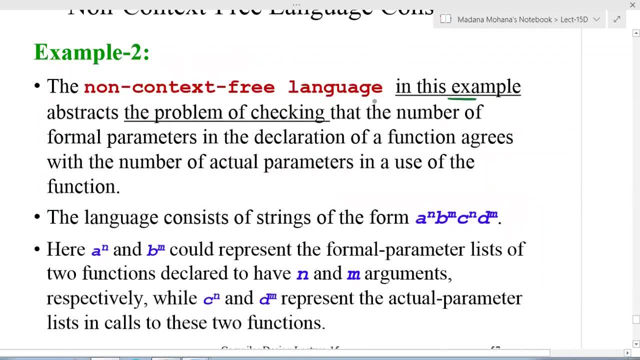 Then the second example. the non-contextual language in this example abstracts the problem of checking number of formal parameters in the declaration of a function. agrees with the number of actual parameters in a use of the function, In this case the language consisting of a string of the form. 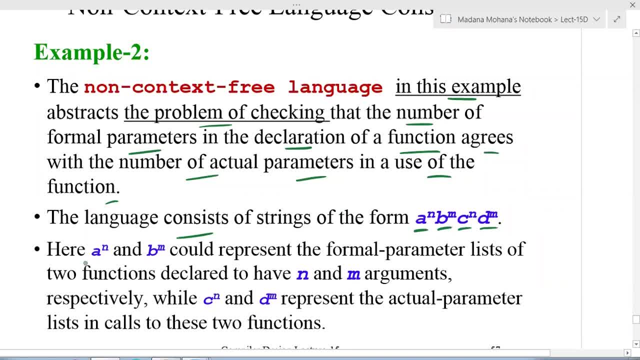 A power n, B power m, C power n, D power m. Here A power n, B power m could represent the formal parameter list of two functions declared to have n and m arguments respectively. Then, whereas C power n and D power, n represents the actual parameter list in calls to these two functions. 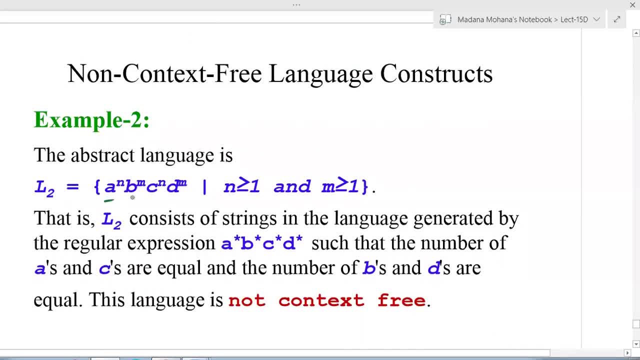 Now the language for this is L2- equal to A power n, B power m. C power n, D power m. Here you can see, for first and third the power is repeated, then second and fourth the power m is repeated, where n greater than or equal to 1 and m greater than or equal to 1.. That is L2 consists of strings in 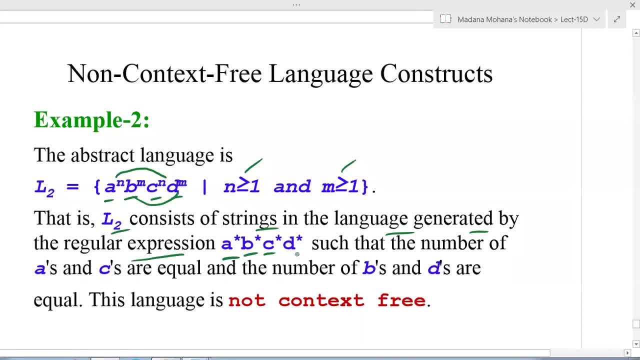 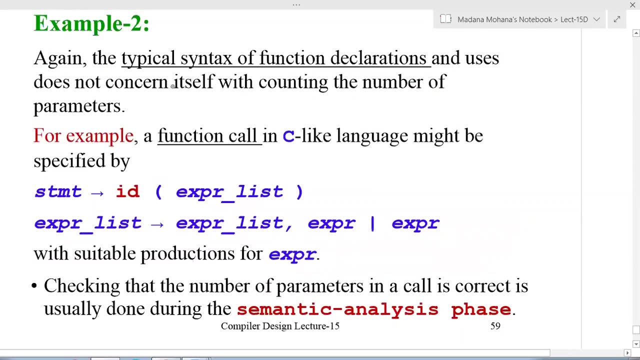 the language generated by the regular expression A closure, B closure, C closure, D closure, such that the number of A's and C's are equal and the number of B's and D's are equal. This language is not context-free language, So in this again, a typical syntax of the function declarations and uses does not concern itself with 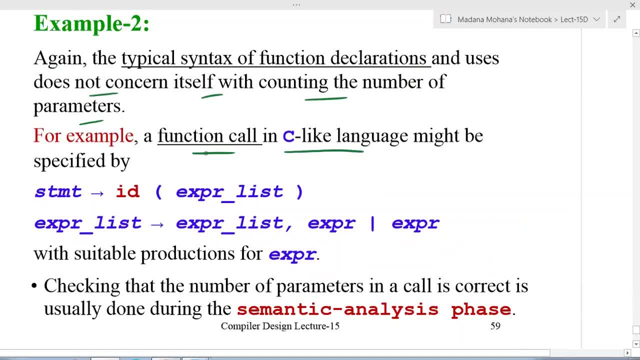 the counting the number of parameters. For example, a function call in C language might specified by statement equal to id, then expression list, where expression list equal to expression list, comma expression or expression with the suitable productions for expression. Checking that the number of parameters in a call is correct is usually done during the semantic analysis phase. 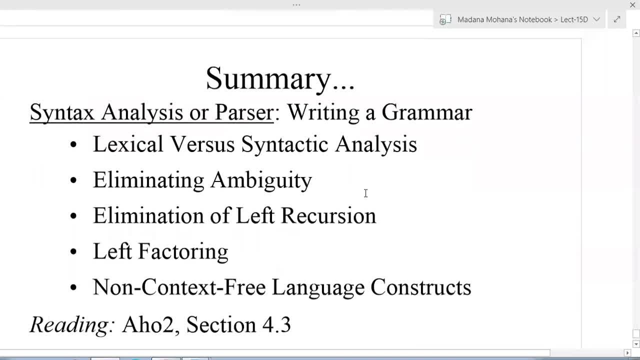 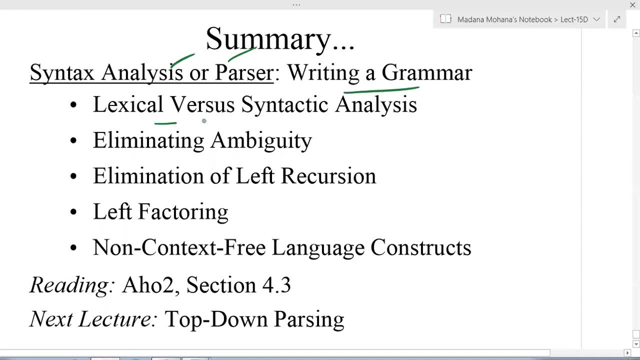 same as previous example, The third phase of compiler. now coming to summary of this lecture. so here, as part of syntax analysis or parser writing a grammar, here we discussed about lexical analysis versus syntax analysis, then eliminating ambiguity using the two methods: disambiguity, rule and precedent, and associative 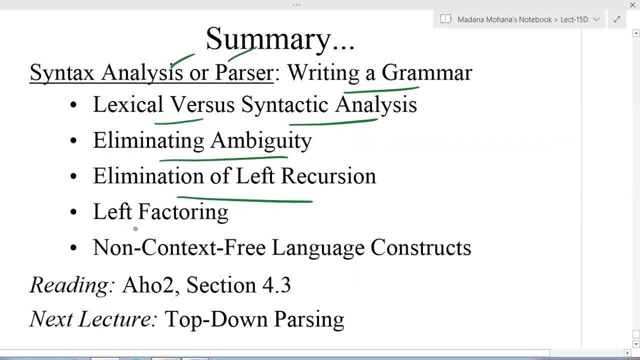 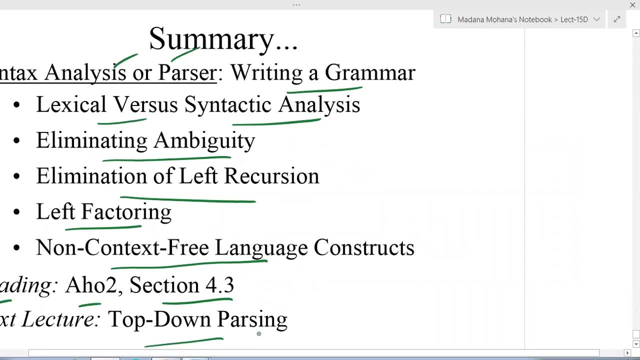 operators, then elimination of left recursion, then left factoring, then non-contextual language constructs. For this lecture the reference is a how to second edition section 4.3. So next lecture we will start with the first type of parser. have done parsing. Now I stop here.